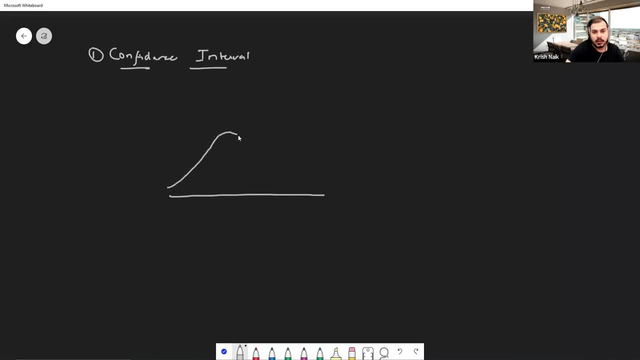 suppose I'll say: okay, this is my distribution and this is how my curve look. okay, this is how my curve will look. okay, just tell me what will be the empirical formula. this is a Gaussian distribution. what is the empirical formula? everyone- I hope everybody- remembers the empirical formula. 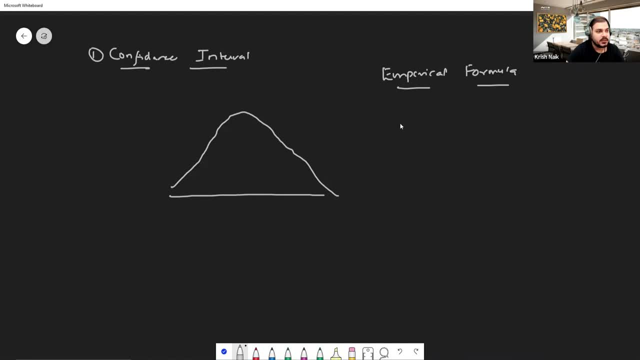 within the first standard deviation, how much data is basically present? within the second standard deviation, how much data is basically present right now? suppose, if I say that within this particular distribution, I want to define some 95% confidence interval, Okay, 95% confidence interval, then what does this basically mean? okay, I want to define some 95%. 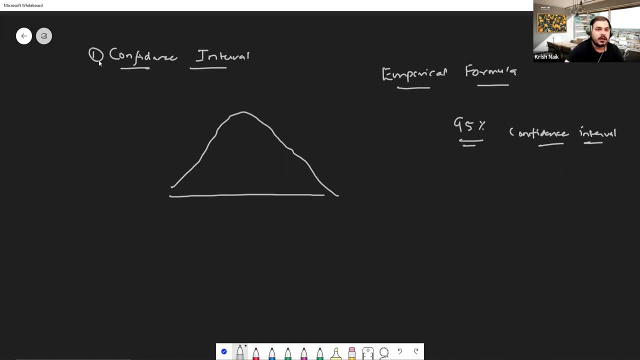 confidence interval. okay, and these all are used in hypothesis testing. I'll talk about it, how it is used. okay, hypothesis testing. now if I say, okay, I want to, I want to basically come up with something like 95 percent confidence interval, how will I do it? okay, now, just imagine over here, guys, if I say: 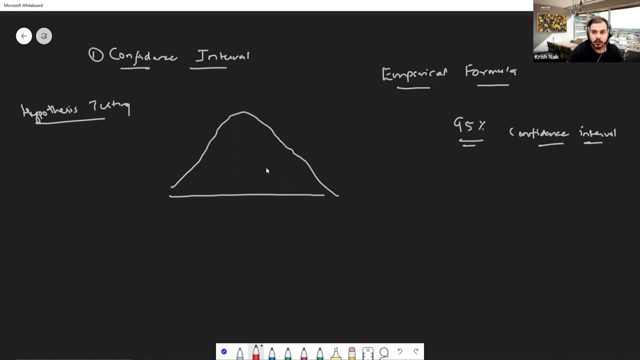 this entire, this entire distribution is my data. okay, and you know what is empirical formula like 68, 95 and 99, right? so this kind of distribution, I hope everybody knows that- basically means within the first standard deviation, 68 percentage of the entire data will be present in the second standard. 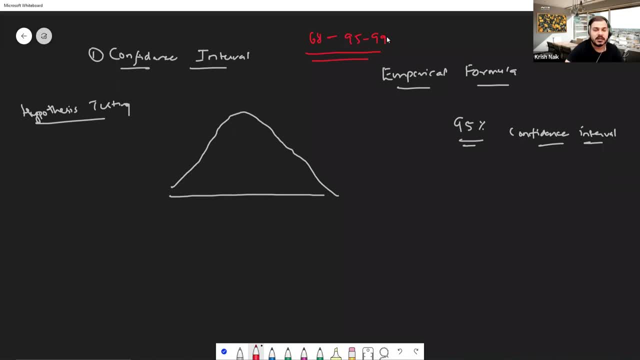 deviation, 95 percentage of the entire data will be present in third standard division. within the third standard division, 99 percentage of the data will be present. right Now, let's take this, this 95 percent- okay, 95 percent- of the um which is basically present. 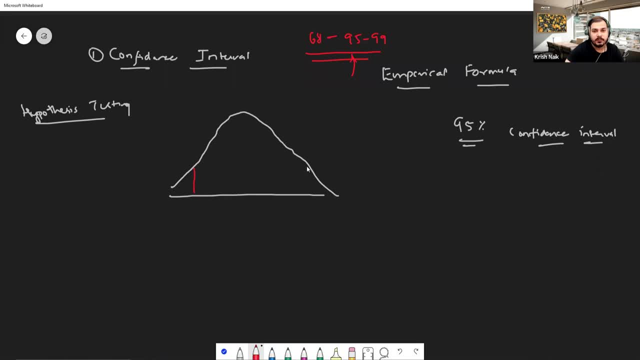 within our second standard division, suppose, if it is this one, this is my 95, this is my 95. okay, so this entire confidence interval from here, from here, which is my mean, and if it comes within this range, any values, I can definitely say that, okay, it is 95, confident, uh, we are confident that it is. 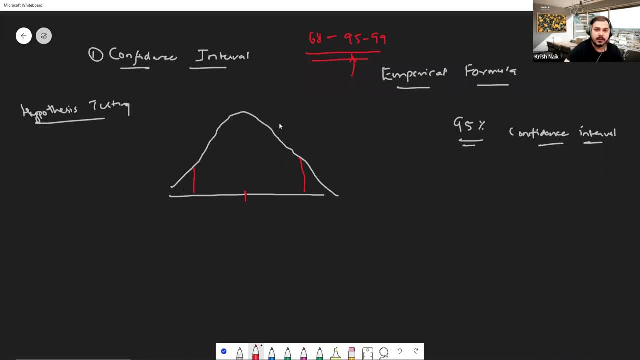 this much in this region. it is 95 percent. it is falling. if it follows, see over here. if I say 95, okay, then how much this will be and how much this will be. guys, tell me how much region this will be and this will be right. tell me, guys how. 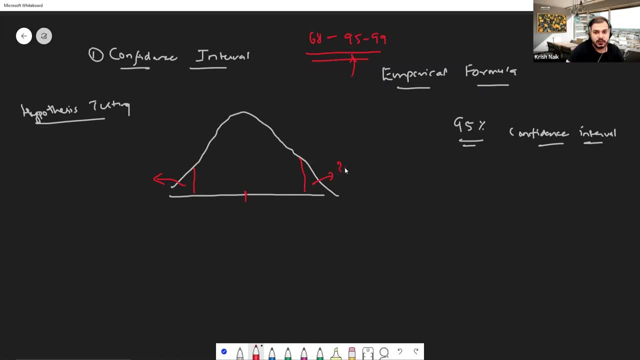 much. it will be 2.5, right. so this will be my 2.5 percent and this will be my 2.5 percent, okay, and this entirely will be 95 percent. right now. why do I say 95 percent? because see most of the points in. 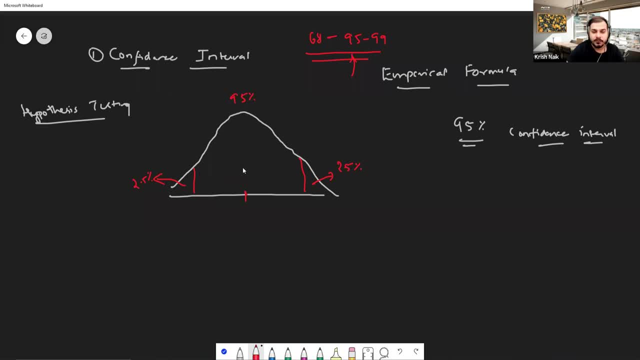 our distribution will fall over here. okay, will fall over here. now one very important point that I really don't start. okay, what is p value? in my previous session I have defined what is p value. guys, suppose if I say that my p value of a specific point over here is somewhere around, p is equal to 0.8. what does this? 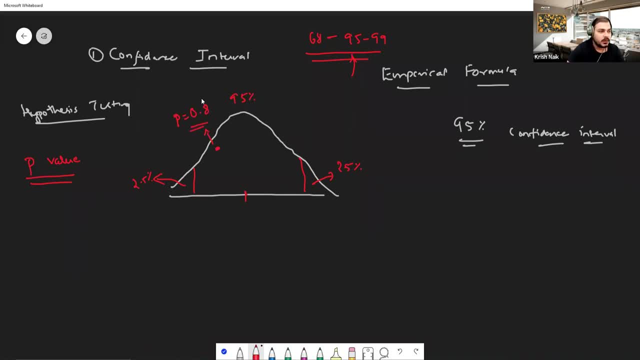 basically mean. I told you guys in our previous session: okay, what does this p is equal to 0.8 mean. what does this p in my previous session look like and what is it equal to 0.8? I told you guys- anybody who remembers anybody, because i i told you one, one, one specific definition of this p value. this basically tells: 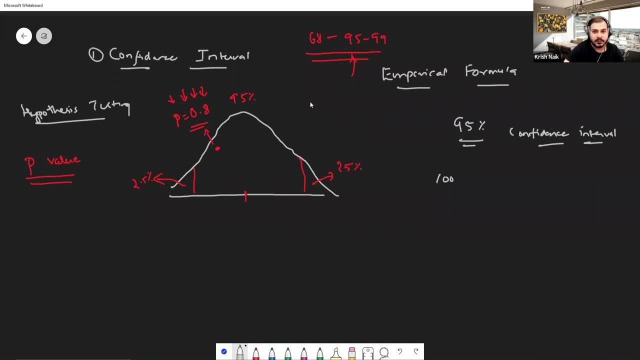 us that suppose if I perform hundred- suppose if I take this example: okay, suppose this is my region of pressing my mouse button. like this right, we have our laptop mouse which looks like this: okay, comes somewhere over here. like this right, If I say that at this point of time, p is equal to 0.8.. 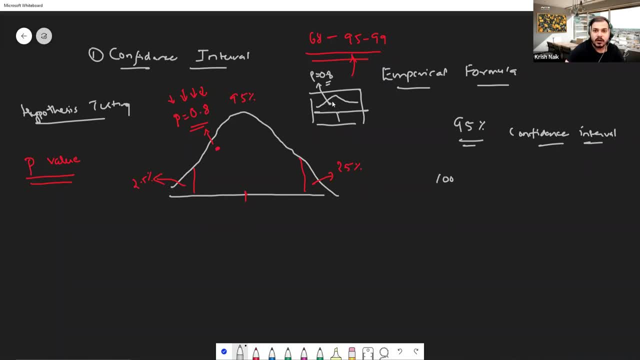 And this basically says that, out of all the touches, out of all, suppose, if I touch 100 times in this particular region, 80% of the time we will be touching here. OK, 8 times, 80%, not 8,, guys, 80%, 80, because it is 0.8.. 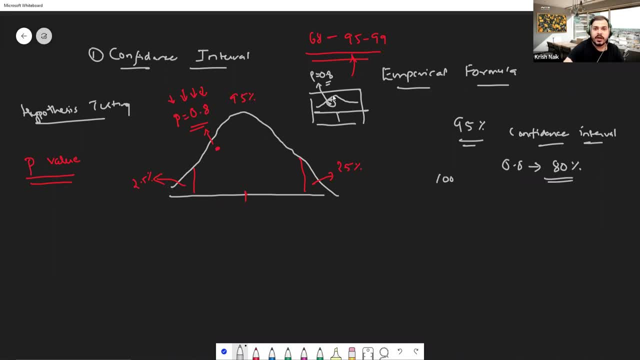 0.8 is nothing but 80%. OK, So 80% of the times. Again, let me draw it in a bigger way, guys. OK for you all. Suppose this is my entire mouse. OK of my laptop. 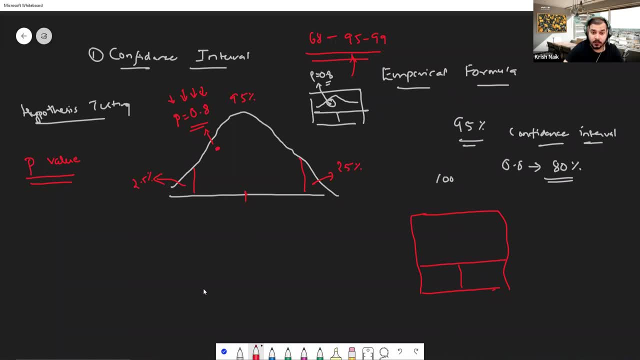 And here I'm actually drawing this, OK, And probably this is my entire distribution. OK, If I say over here, the p value is 0.8, this basically says that out of every 100 experiment, or out of every 100, touches 80% of the time. 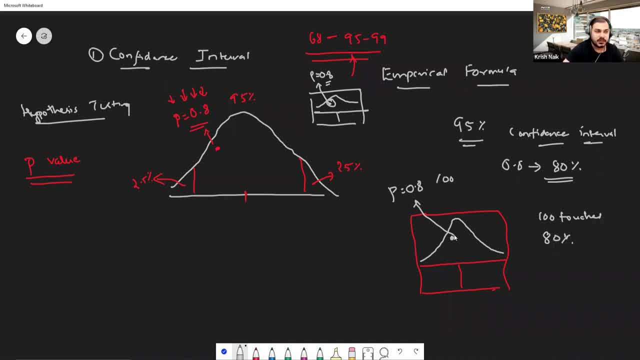 or 80 times the touch was here. OK, Suppose over here, if I say p is equal to 0.01.. What does this basically say, guys, If p is equal to 0.01,, anybody? If p is equal to 0.01, tell me, tell me, tell me quickly. 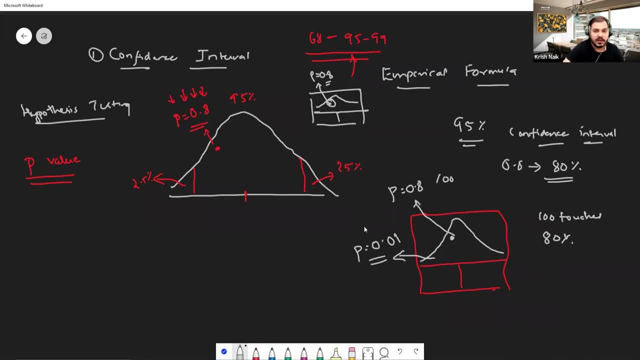 That basically means, out of every 100 touches, I will be touching one time over here. OK, So something like this: Now, if I say p is equal to 0.01.. Tell me whether this p is equal to 0.01,. 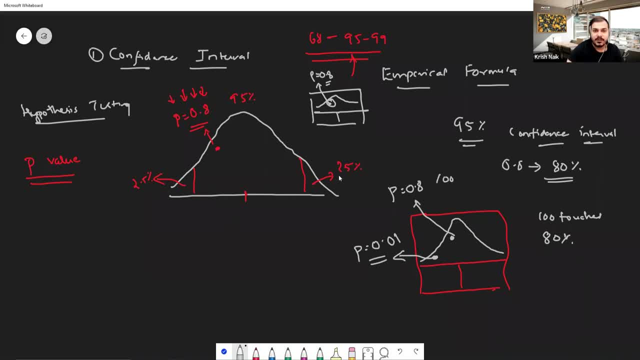 whether it will be falling in this 2.5 area- 2.5 percentage area- or it will be falling in this 95 percentage confidence area. Tell me guys In the 2.5 area, right, It is very, very simple. 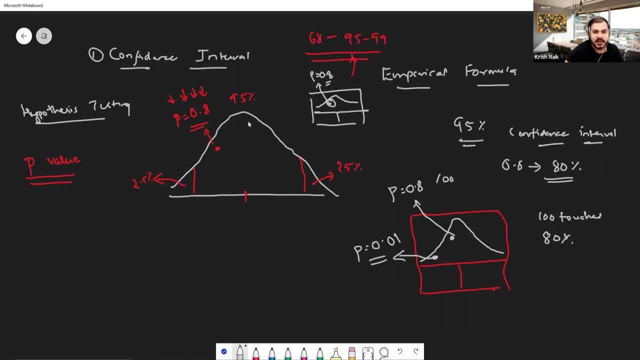 In the 2.5 area. right, Always remember this entire region. if I try to split this like this, OK, this entire region is symmetrical to this particular region. OK, This particular region. That basically means in a Gaussian distribution: 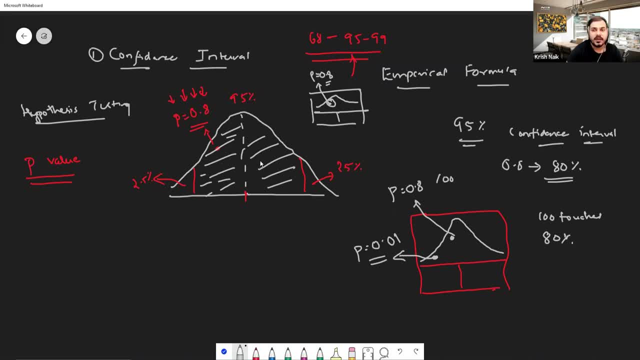 the amount of data that is present over here is equal to the same amount of area that is present over here. Now, guys, is my voice breaking? Guys? I don't think so. my voice is breaking, right, Ritesh, please have a look onto your internet, OK. 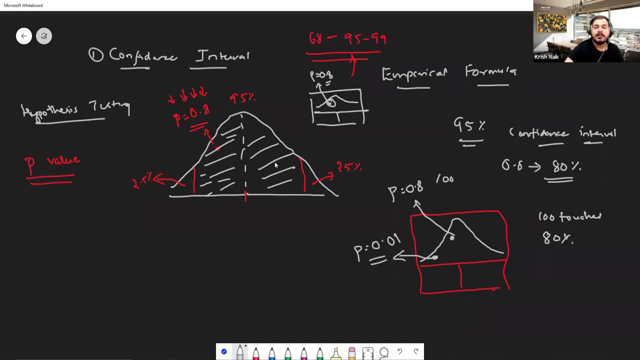 Perfect. Now, when I say that this area is symmetrical to this area, I can definitely say that any value, any value that is between this to this, This to this, actually falls in the confidence interval of 95%. OK, And any values that fall outside of this. 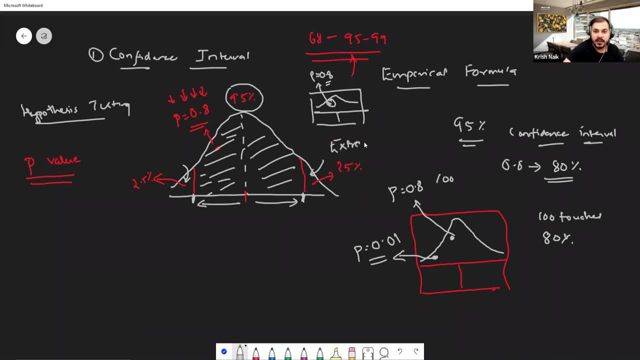 is basically in my extreme ends. This is called my extreme ends, OK, Extreme ends. I'll tell you why this is very, very much important. OK, Now let's I told you right This p-value, whatever we say. suppose, if I say p-value is 0.8,. 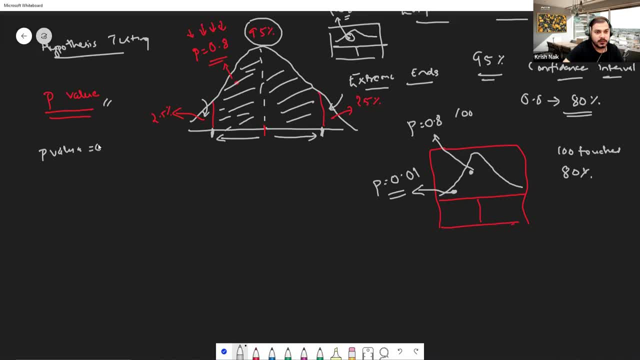 p-value probably. OK, I can keep it as 0.05, right? This is called as significance value. I'll talk about it, why it is important everyone. OK, This is called as significance value. OK, Always remember this, OK. 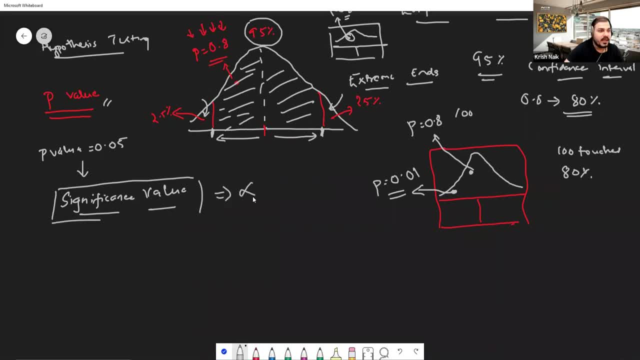 P-value. we can say it as significance value. It is also denoted by alpha. you know It is denoted as alpha also and it can also be told as a p-value, But most of the time we say it as significance value. 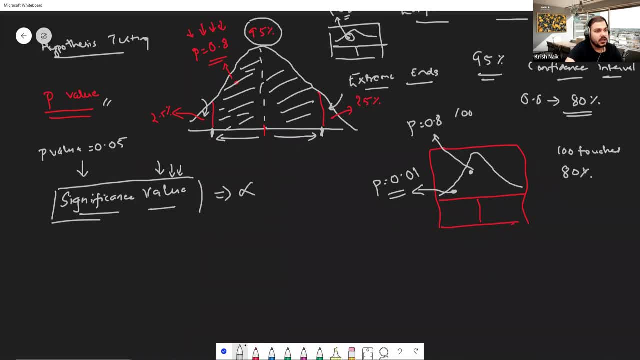 OK. So it is very, very much important, guys, Always make sure that you always make sure that you basically remember these terminologies, because it is important, because it will be coming some or the other way, always. OK, Now where exactly it is used. 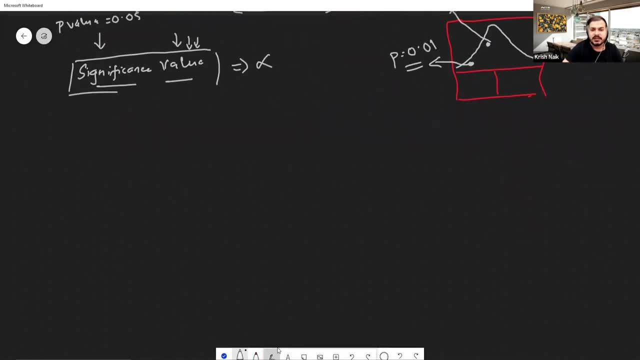 OK, Suppose let's take a very good example. I hope you got an idea of hypothesis testing. Yeah, Yeah, Yeah, Yeah, Yeah, Yeah, In hypothesis testing what all things will be there. guys, Tell me First what all things will be there. 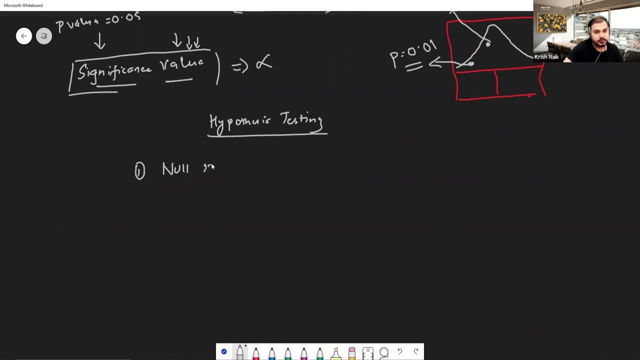 What all things will be there in hypothesis testing. guys, Null hypothesis, right. Then we also define our alternate hypothesis. OK, Then what we do? We collect evidences, right, We collect the evidences. Collecting evidences is, in the case of law, law example. 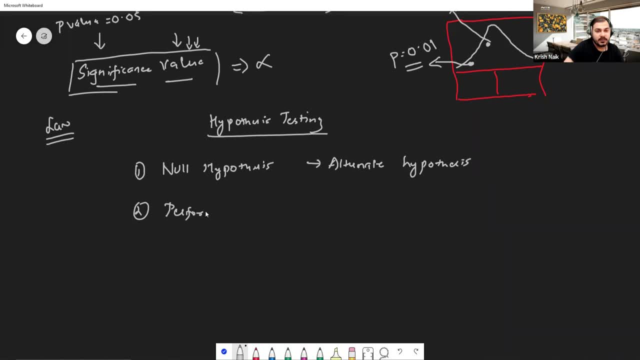 that I gave you. But here we will perform some kind of experiments. Perform some kind of experiments, OK. This experiment is usually performed with this some significance value. Here I'll say that my significance value will be 0.05, OK. 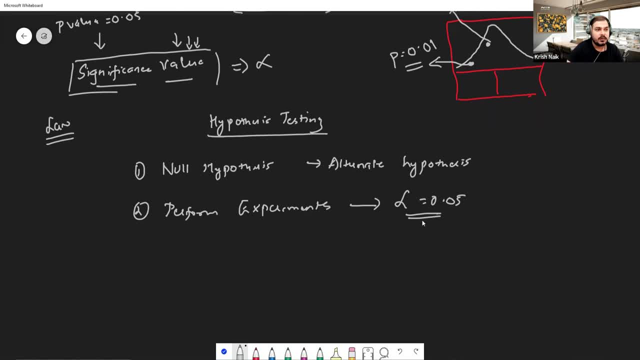 I hope everybody is understanding Here your significance value, it will be there some alpha value. It will be there with 0.05.. And we'll perform some experiments. Now, what kind of experiments can be performed? There are various kinds of experiments. 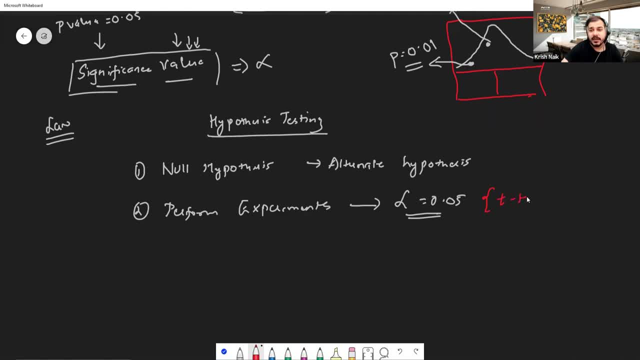 which I'll be discussing today. OK, There will be something like t-test, z-test, chi-square test. OK, There will be ANOVA test. A lot of different, different tests are there. OK, We will discuss about this. OK. 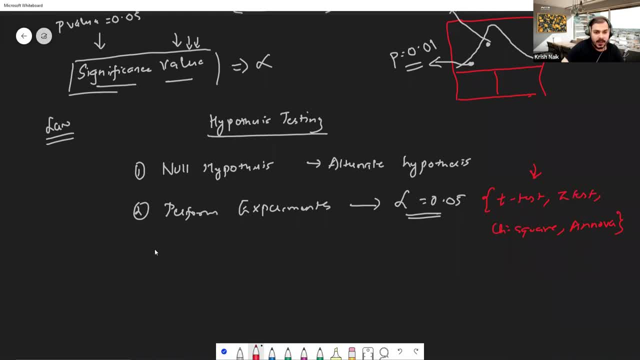 What test is used for what purpose? OK, And then we come to the third part. OK, OK, OK, OK. After performing the experiment, we get some value And, based on the significance value, what we do if it falls. 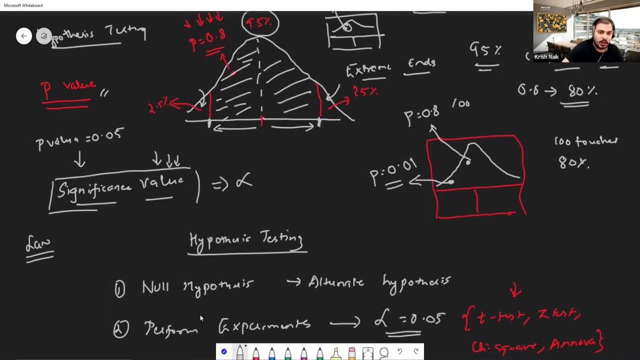 if it falls in this extreme area, if the value or output that we get if it falls in this extreme area or in this extreme area, what we do? We basically reject it. OK, What we do? We basically reject it Because, see, based on this alpha value. 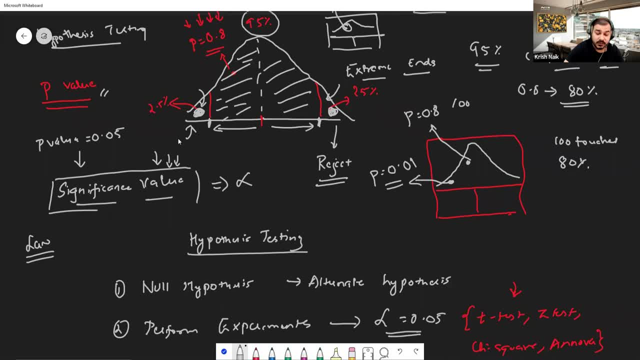 it should be coming over here If it comes in this region and this region. Now you may be thinking, Krish, should we take alpha values 0.05 only? No, It depends on the domain knowledge. right, It depends on the domain knowledge. 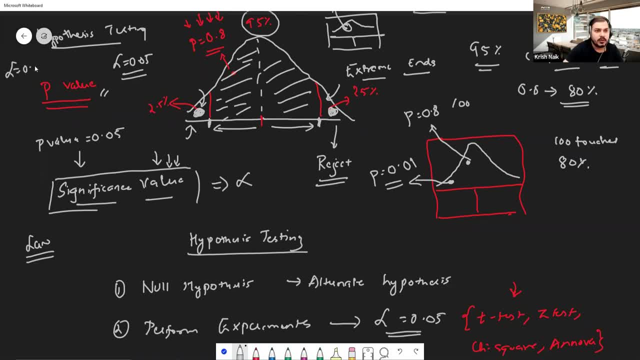 If my area is small, I may take an alpha value 0.01.. I may take much more smaller. Who decides this? A domain expert decides this. OK, But by default, many people go ahead with. alpha is equal to 0.05.. 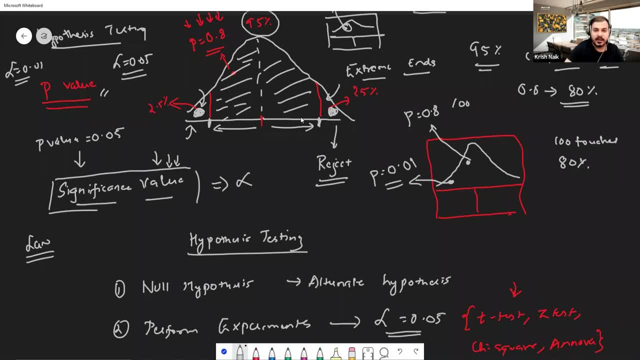 Now understand over here. when we perform the experiment and suppose, after performing the experiment we get a value from a z-test, we get a value that falls here or here In the extreme ends- this is my extreme end. If it falls over here, we reject the null hypothesis. 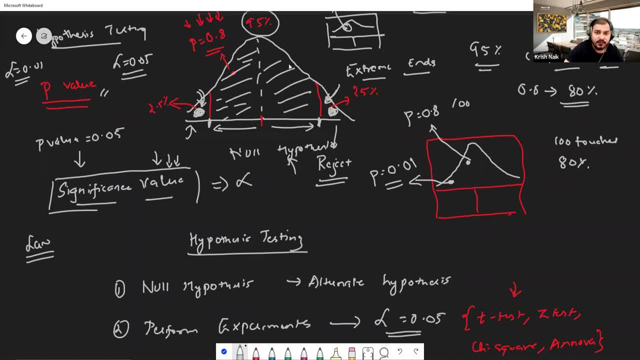 We reject the null hypothesis And anything that falls in this 95% confidence interval. if your alpha is 0.05, then obviously your confidence interval will be 95%. If your alpha is 0.01,, what will be your confidence interval, guys? 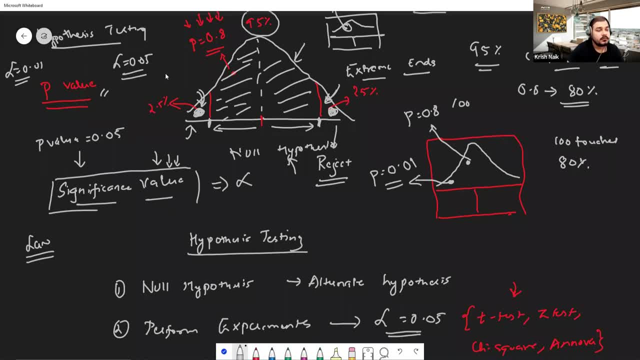 What will be your confidence interval If alpha is 0.01,? what is your confidence interval? It will be 99%, right? I hope everybody's understanding It will be 99%. OK, Now understand over here with respect to this particular confidence. 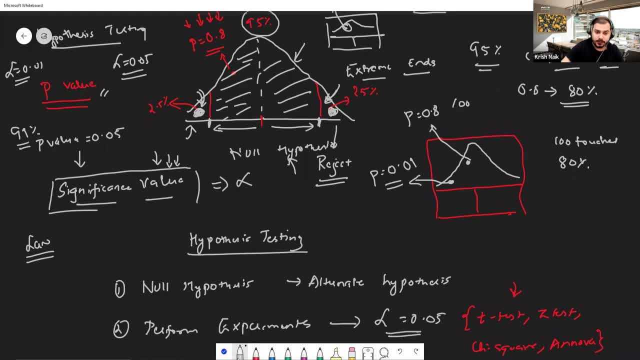 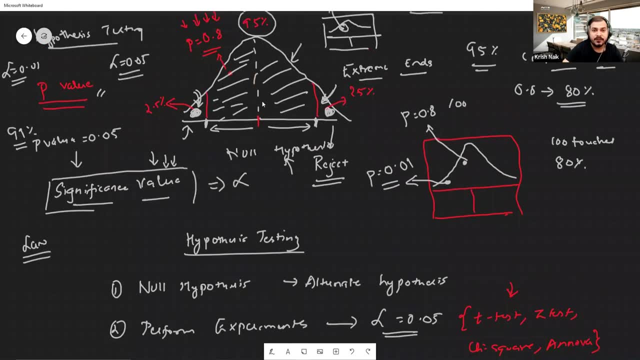 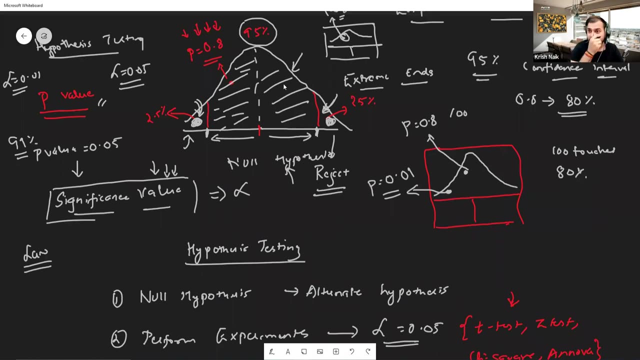 interval. if my data, whatever experiments I have actually performed over here, whatever experiments I have performed over here and based on this experiment, if that value falls over here, OK, then we are going to accept the null hypothesis and reject the alternate hypothesis. 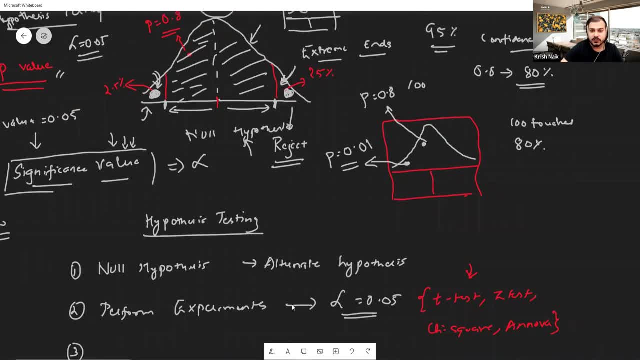 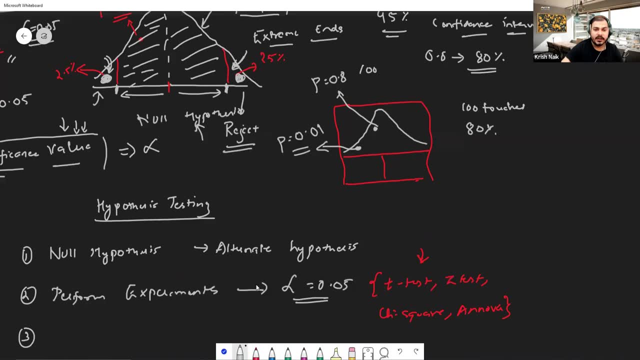 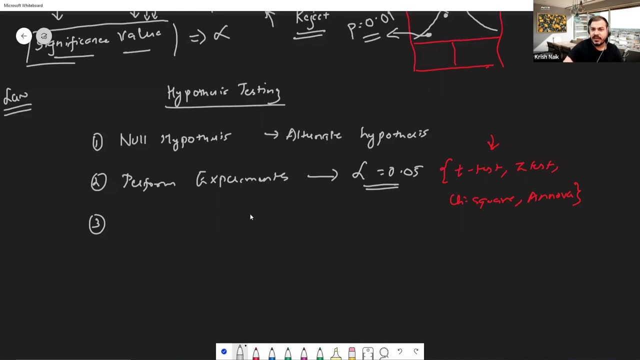 It is very, very simple, guys. See if my values, I'll just write it down over here. If after the experiment, I'll write down over here after the experiment. OK, if the value, whatever value, whatever test value, I'll write over here whatever test value falls. 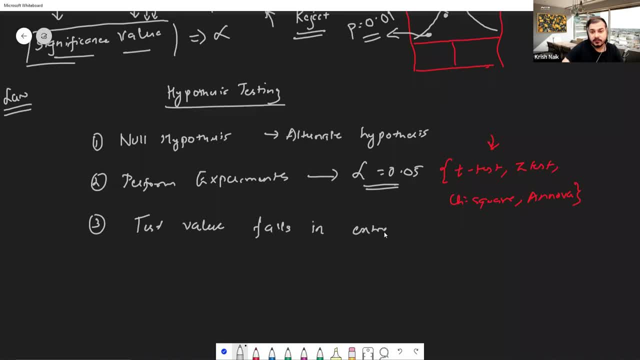 in extreme end. if it falls in extreme end. what we have to do, guys, We reject the null hypothesis. and we, what we do, We accept the alternate hypothesis. I'll talk about it, guys. I'll give you a very good example. 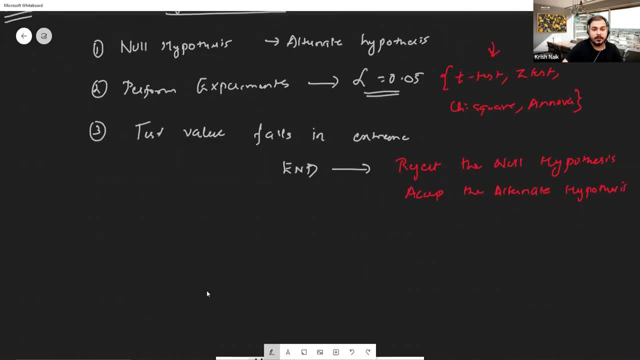 OK, Don't worry. OK, Suppose if the test value falls in confidence interval. Now how this confidence interval is defined, Based on your significance value. If your significance value is 0.05, your confidence interval will be 95%. OK, 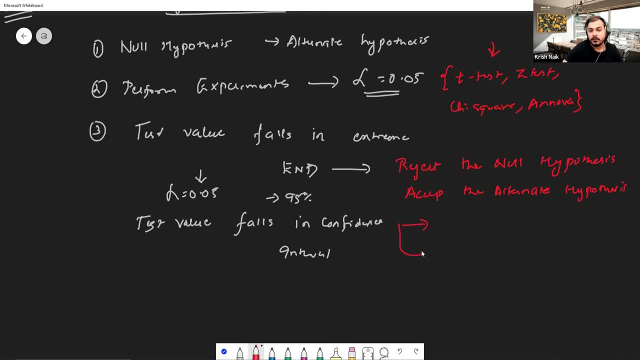 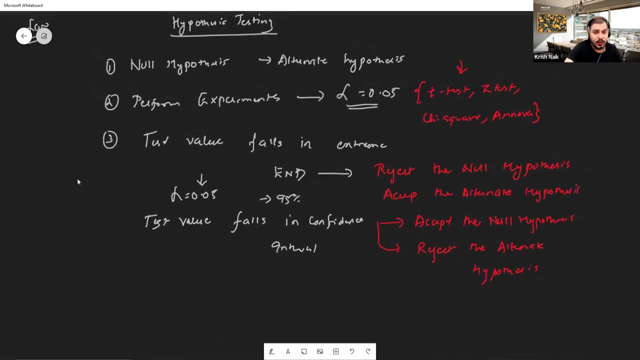 At that particular time, what we do. We accept the null hypothesis and we reject the alternate hypothesis. Guys, is it clear? everyone, Yes, Guys, very, very simple What I'm just? I'm just saying that I'll talk about it. 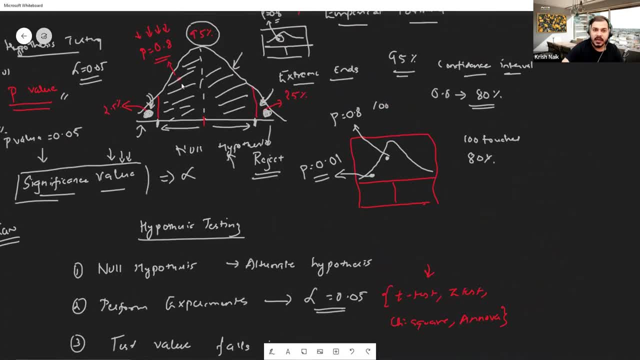 How you will be able to get all of this. I'm just saying that if, after the experiment, if your value does not fall in this region, if your value does not fall in this region, then what we are going to do, We are just going to that- basically means your value falls into the extreme end. 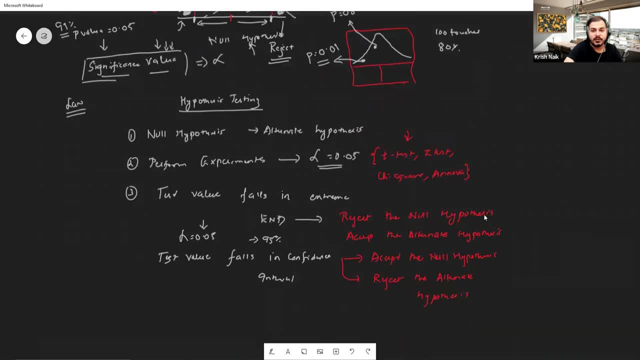 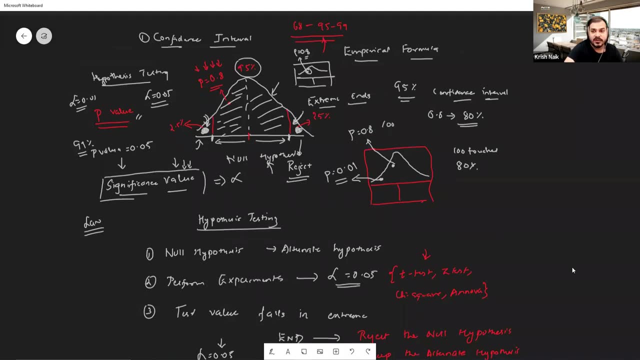 Then what we are going to do? We are basically going to reject the null hypothesis. We're going to accept the alternate hypothesis, Suppose if it falls inside your this specific region in 95%. then we are just going to accept the null hypothesis and reject the null hypothesis. 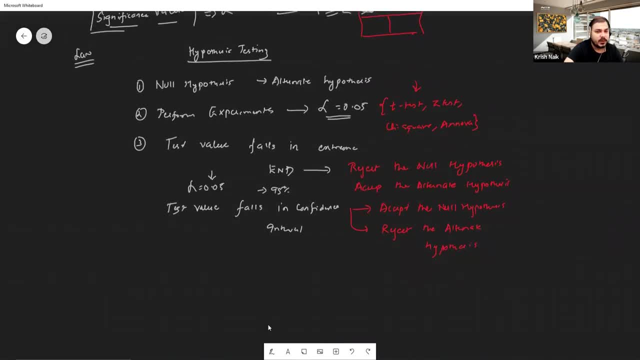 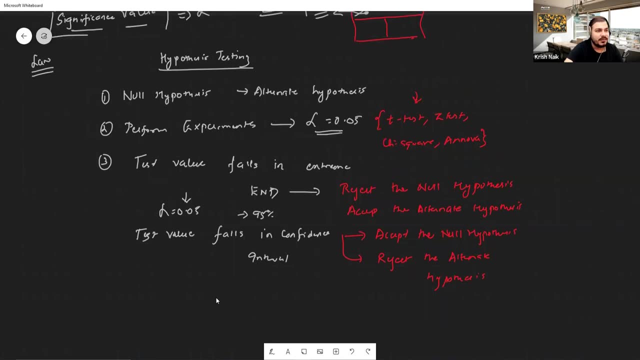 Alternate hypothesis: OK, Alternate hypothesis. I hope everybody is able to understand right? Very, very simple, very, very easy right. I've not done anything much. OK, I've not done anything much. Very, very simple things. 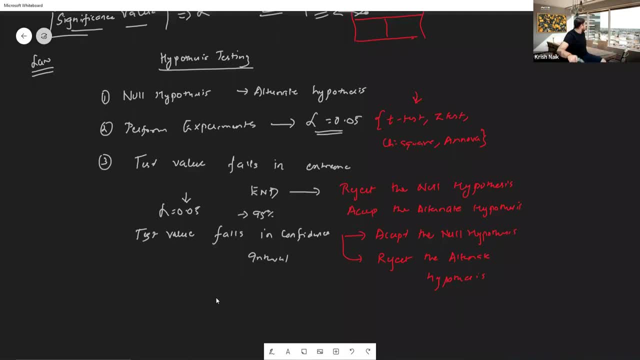 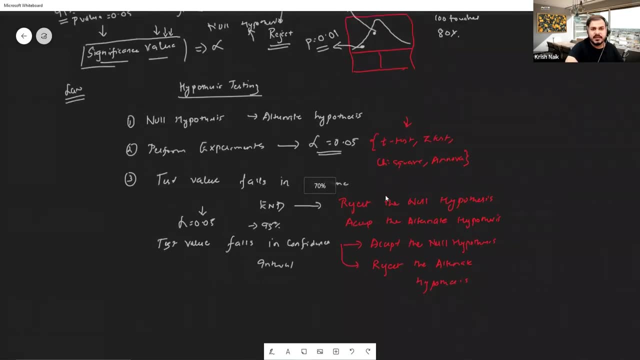 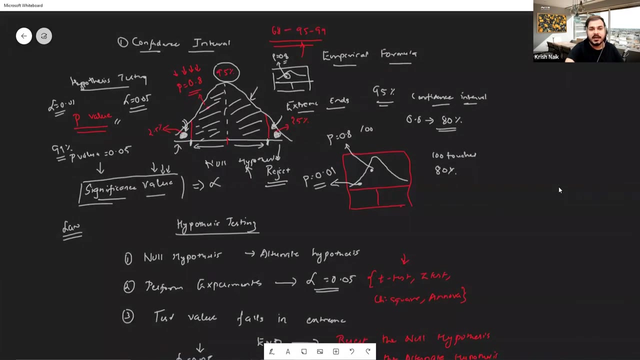 We have just understood something. OK. I hope everybody is able to understand it. Very simple. I think you will never find this kind of explanation, guys. Have you Have Anybody who tried to understand before what is confidence interval? and all right. 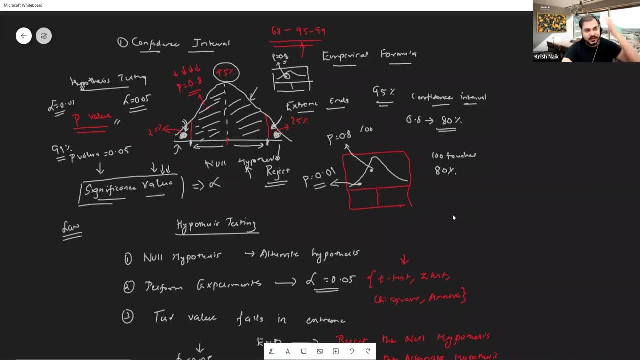 No, I guess Just understand. Confidence interval is not 95%. again Again, I told you guys how do we define confidence interval. We basically say: based on our alpha value. Suppose tomorrow my domain expertise says alpha value take it as 0.06.. 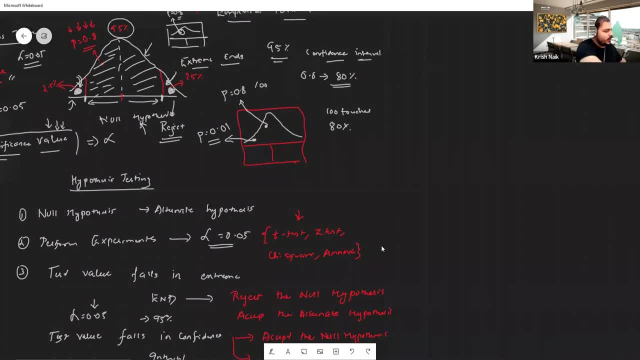 Then what will be my confidence interval? 1 minus 0.06 is how much? 1 minus 0.06 is how much? 1 minus 0.06 is what? 1 minus 0.06 is what 0.06.. 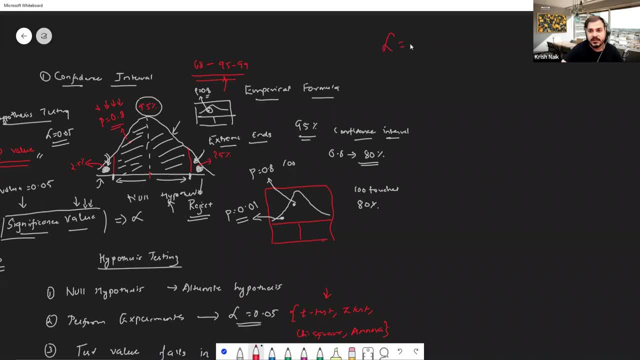 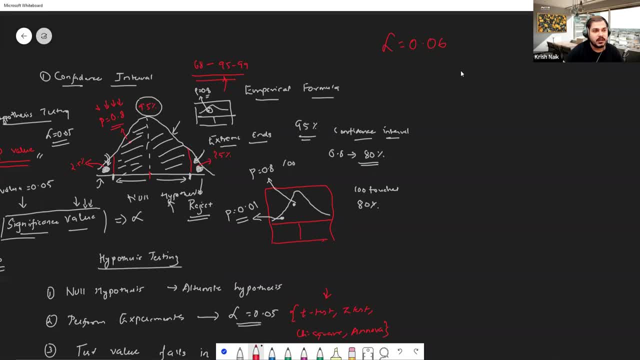 0.06.. 0.06.. 0.06.. 0.06.. 0.06.. 1 minus 0.06 is how much 6%, Right? So my confidence interval will be 94%. Okay. 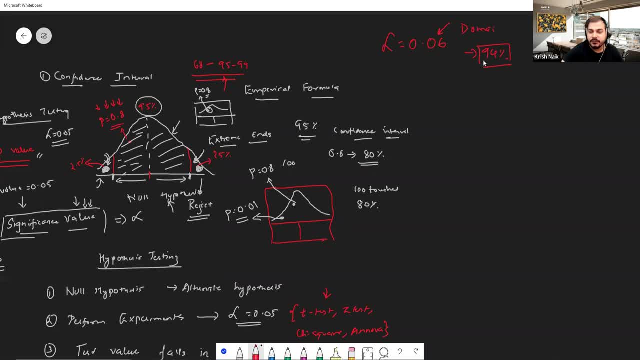 Understand in life's way How we define this alpha value. This is defined by the domain expertise, So we don't have to worry much over that. If you don't know anything, just take the alpha value as 0.05.. That basically means I want it in my 95 confidence interval. 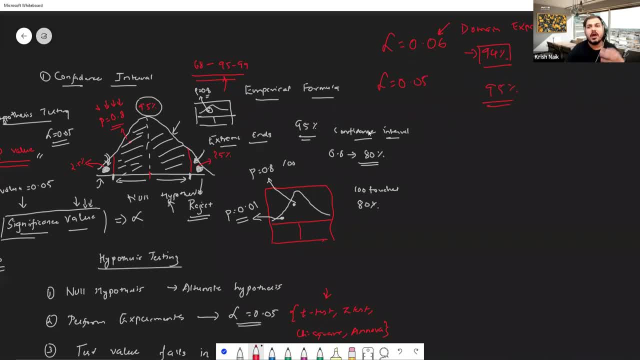 Okay, I hope everybody has got understood now. Now let's solve a specific problem. Okay, And remember, this is very much important. Okay, In hypothesis testing. hypothesis testing is the most important question that is asked in statistics. Everybody is able to understand why I'm focusing more into this. hypothesis testing is the most 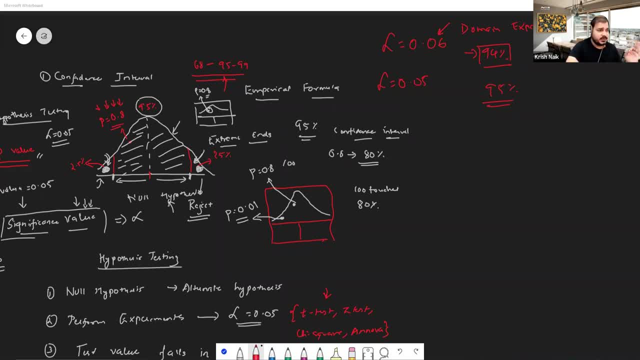 important thing. Okay, In statistics, anytime, any interviewer will try to confuse you in this, And if you're able to explain them. many people have confusion with respect to P value. What is this P? You are looking like a scientist will be after my 0.0, they don't know about this confidence. 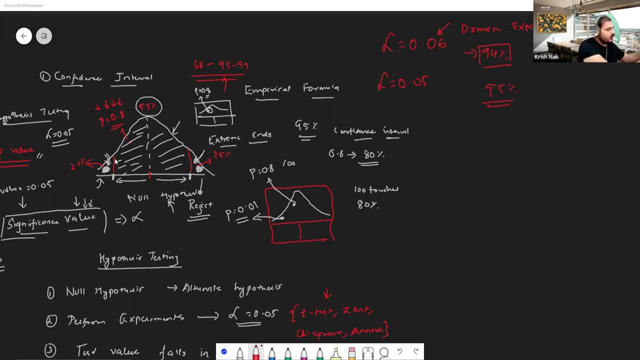 interval. Okay, That is the reason why I'm telling you to focus on this. Now, let's go ahead and solve a specific problem. Shall we solve the specific problem. Shall, we solve a specific problem. Okay, One more thing that I really want to talk about. 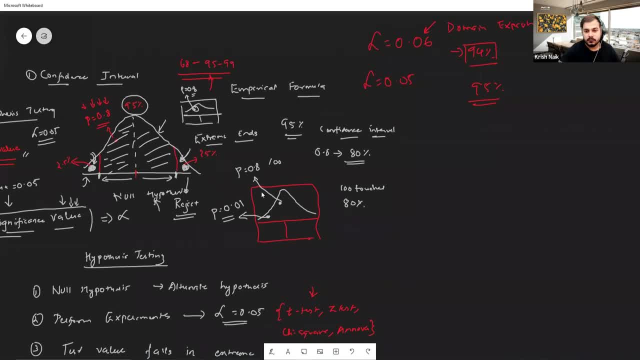 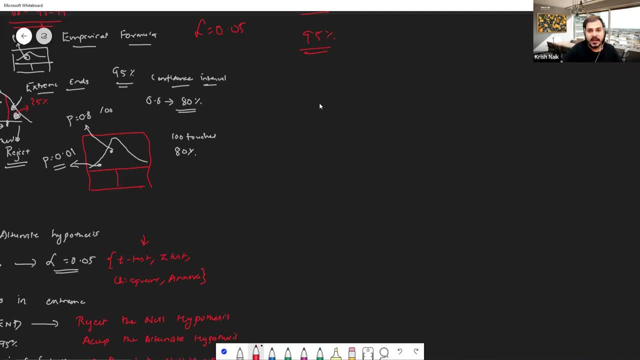 The other concept that I really want to talk about is Now all this kind of tests or experiments that we perform form guys, it can be defined as one tail test and two tail test. okay now, one tail test and two tail test. let's define what. what exactly it is? suppose this is my normal distribution. 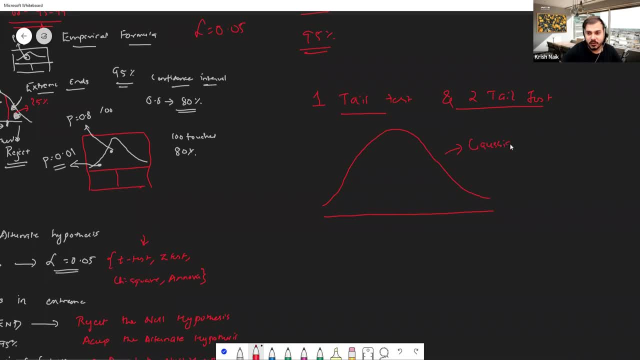 guys, this is my gaussian distribution. okay, don't fear that, chris. no, you have not drawn the diagram properly, so i'm writing an example over here. so this is my gaussian distribution. now, when i say 95 confidence interval at both the side, i can draw like this: this will be my 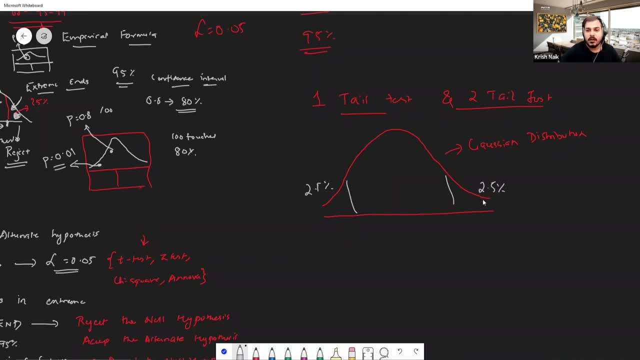 2.5 percent. this will be my 2.5 percent now in this guys. okay, understand one thing. suppose this is my mean value. okay, suppose i want to perform one experiment. suppose i say that my population. suppose i uh in my population. uh, i see that my population is having a mean of 120. 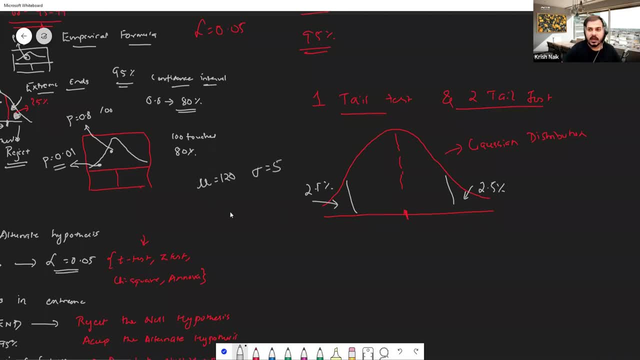 and standard deviation is equal to 5. okay, i, just i. i, i have a population with some n value. probably. my n is 100, okay, and my mean is 120, and standard deviation is 5. okay, now suppose, if i take up a sample of 30? okay, i picked up a sample of 30 from here. 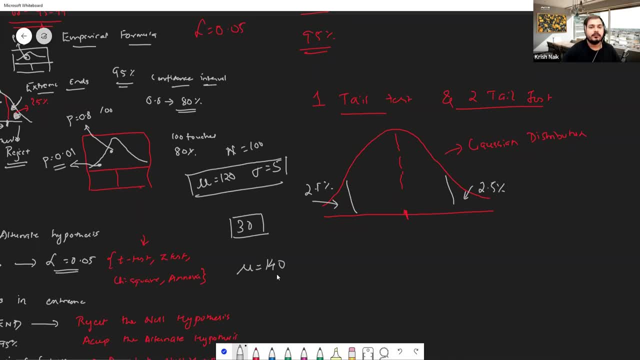 and suppose i say my mean is 140.. okay, suppose i say that my mean is 140. i have calculated this sample of 30 and i found out the mean is 140.. can i say that? can i say that? and probably this sample that i've picked- you know, i've picked up from this- 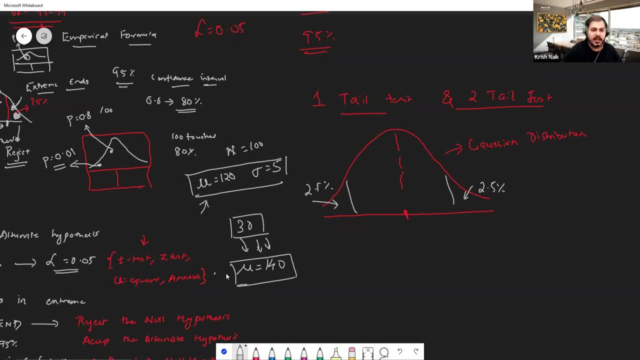 particular population. can i say that the mean of the population and the mean of the sample are same? okay, over here, sorry, okay, fine, i'll. i'll make it as x bar. okay, x bar. can i say that this mean and this x bar are same? okay, so i'll perform an experiment. i'll say that after performing an experiment, after. 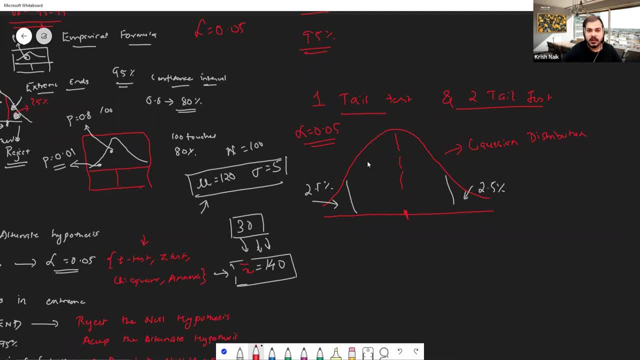 selecting some significance value. if, if that entire area falls over here, if it falls away, what i have to do, guys, if it falls over here, what i have to do, guys, if it falls over here, what i have to- okay, i'll talk about it. i'll talk about now, here, what we 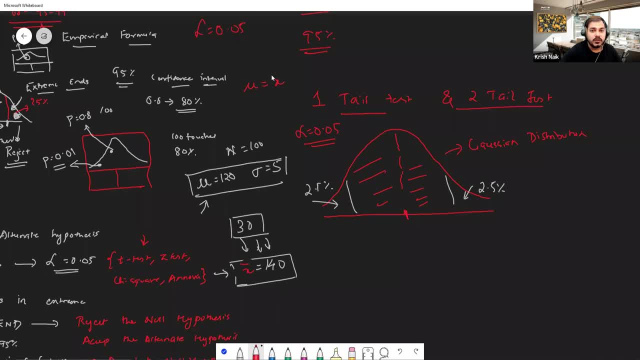 are doing? we are just comparing whether mean is equal to sample mean or not. we are comparing this right, yes or no? we are comparing this: whether this is equal to this, yes or no? guys tell me, yeah, now, when we are comparing this, this x bar may be less than mu. x bar may be greater than mu. 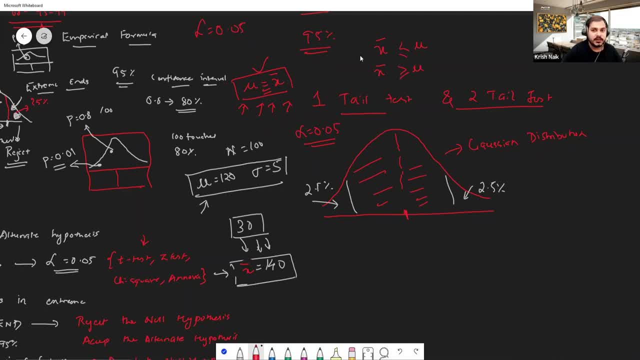 less than or equal to mu or greater than equal to mu. yes, yeah, this, both can be there, okay, and here i'm taking the sigma value, or alpha value, as 95 percent. that basically means my this x bar can fall from this range to this range. do you agree with me? yes, yes or no, everyone quickly tell. 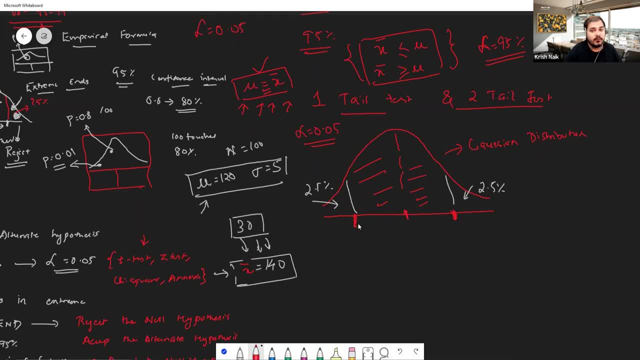 me, do you agree with me whether the x bar will fall from this range to this range? yes, if it falls in this particular range, i'll obviously reject the another hypothesis. i really want my x bar to fall within this 95 confidence interval. now i know my x bar can be greater than. 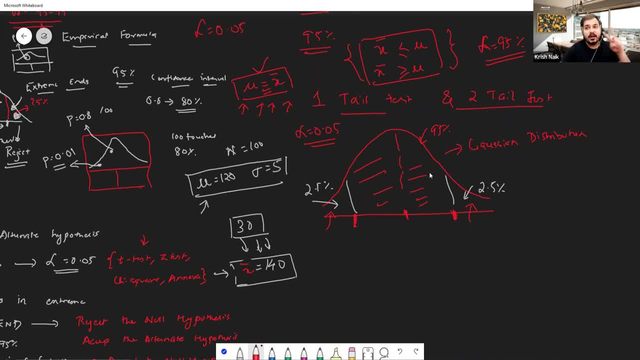 or equal to mu, or less than or equal to mu. so this kind of tests are called as two tail test, because over here your x bar can be less than or equal to mu. it can also be greater than or equal to mu. so let's look at that again. 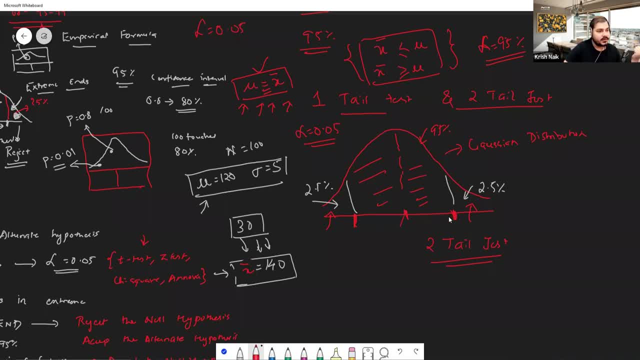 than also. it can also be less than this, it can also be greater than this. so in this scenario, this becomes a two-tailed test. okay, this becomes a two-tailed test. now tell me a guess what will be. one-tailed test: rajesh, rajesh saravan. p value and alpha value are one and the same. 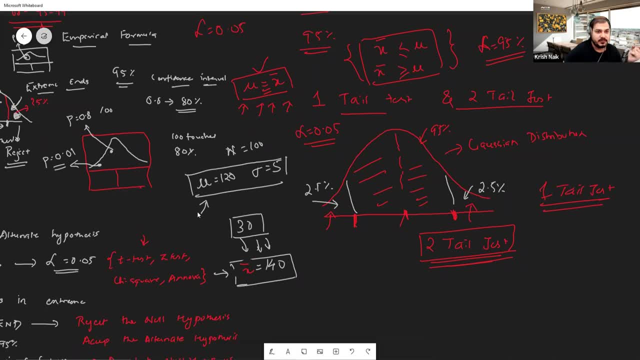 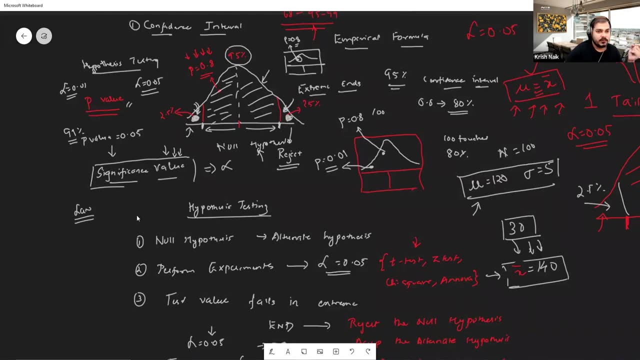 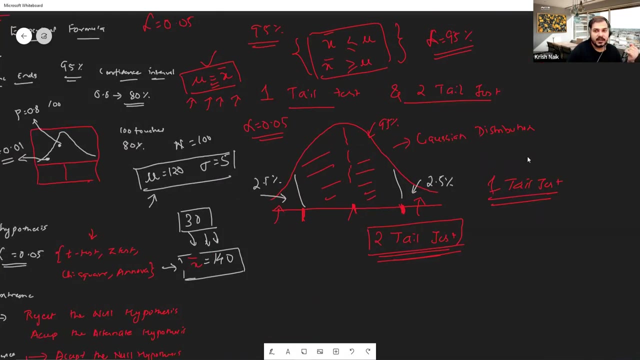 okay, we basically say here i've clearly written right p value and significance value. right, we also say this as a significance value: right p value and significance value. so tell me one example with respect to one-tailed test: what? what will be a one-tailed test? can i say that? 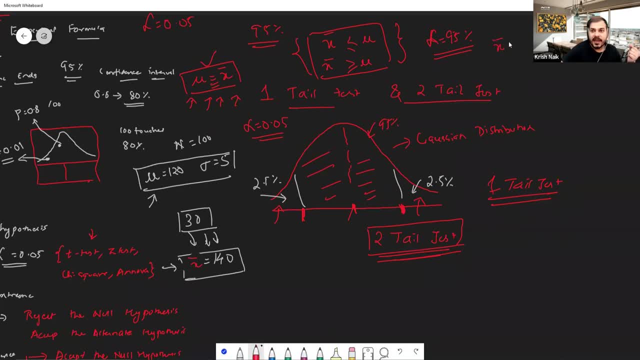 can i say that my x bar, suppose i say, is greater than 140? suppose i want to perform this experiment. then i don't have to worry about this below part, right, i don't have to worry about the below part, i just have to worry about the greater part, so that becomes a one-tailed test. i hope everybody is able to understand. 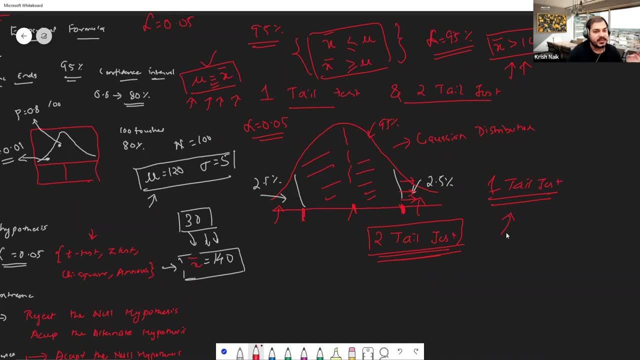 the basic difference between two-tailed test and one-tailed test. in two-tailed test, i told you that, whether my mean is equal to x bar, i have to perform an experiment, and here the scenario may be that it may be less than or equal to mean. it may be greater than or equal to mean. 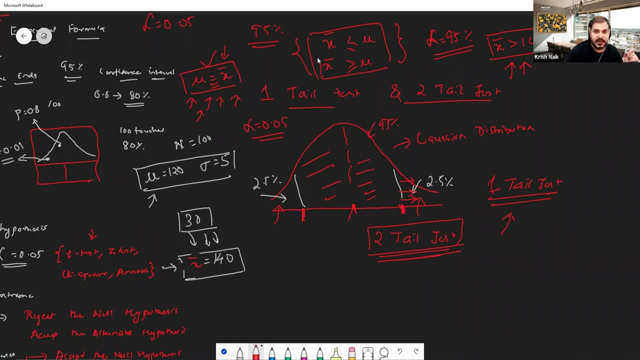 right, it may be less than or equal to mean it may be greater than or equal to mean it may be. suppose if i say greater than or equal to mean- i just want to check this- then it will become one-tailed test. if i want to compare both, then it may become two-tailed. 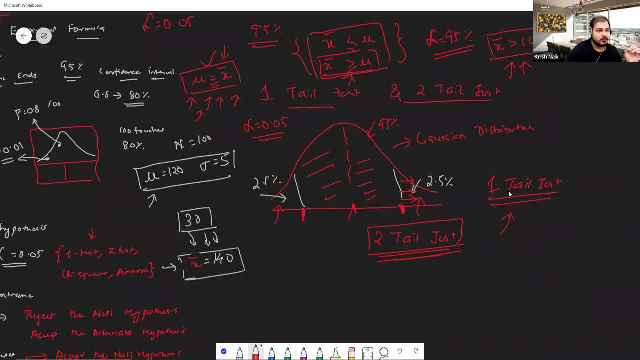 test, krish, are you comparing the mean of both sample and population over a single gaussian distribution? yes, yes, tushar, i'm doing that. okay, so if it involves either one side of the area, okay, from this entirely is considered as one side of area from this particular point. 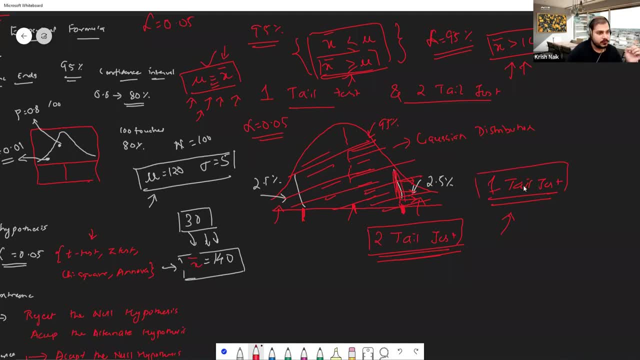 okay, then i will be considering it as a one-tailed test. guys, is it clear or not? yes or no? everybody, i want some answers from you. come on, please tell me. it's very, very simple, guys. right, it's very, very simple what i have done over here. nothing very simple i i have told. 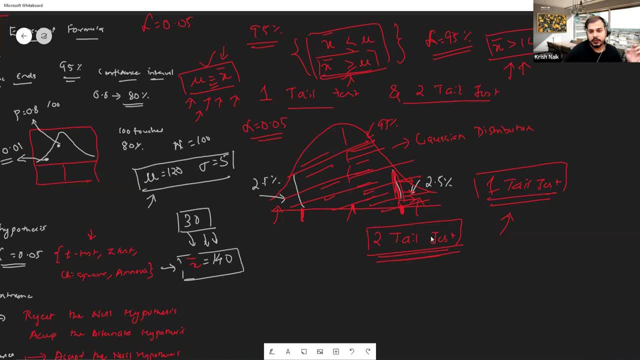 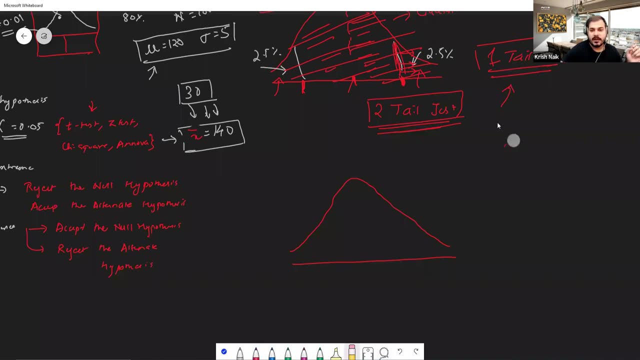 you a problem statement. suppose this is my gaussian distribution: right population, gaussian distribution. suppose my population, my population, suppose my- i'll say my capital- n is 100, my mean of this is 120, my standard deviation is 5.. now what i did? i picked up 30 sample, i calculated the mean. suppose my sorry, here again, i'll write it as x bar. 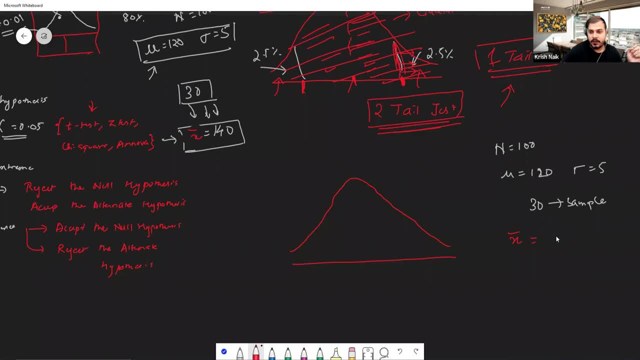 here i've calculated the mean. the mean is somewhere around 140.. now can i say whether x bar is equal to mean, or can i say x bar is less than mean, or can i say x bar is greater than equal to mean? i have to check this three condition now. whenever i check this particular condition, i select some alpha. 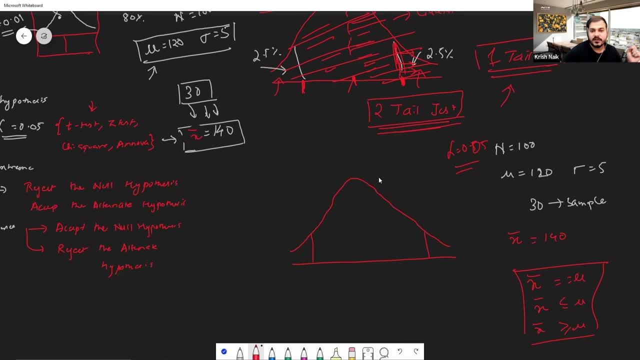 value. so alpha value is 0.05. that basically means i want 95 confidence interval. so this is my 95. now, in this particular scenario, when i cut checking these three conditions, okay, i have to focus on this tail also, in this tail also, so this becomes a two-tailed test. 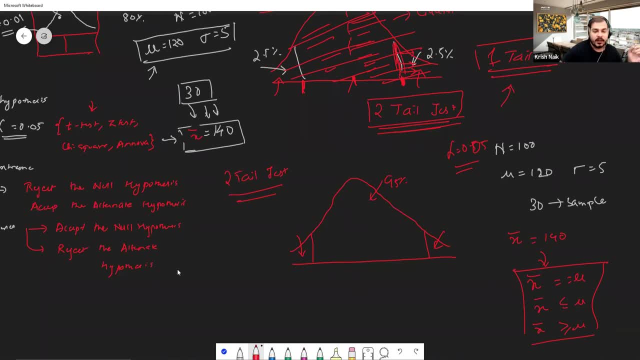 suppose if i say that i just want to check whether my x bar is less than 140 mean, or is it less than 120 mean? so here i'm checking less than right. so less than basically means it will be coming over here. suppose this is my mean right: 120, it will be coming over here. 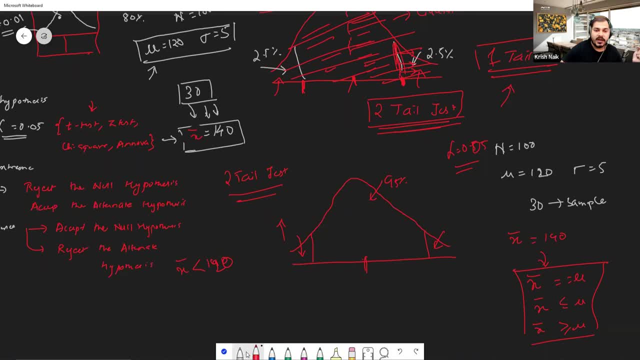 i don't have to worry about this particular part, so this becomes a one tail test. suppose i say if x bar is greater than or equal to 120. i want to check this with respect to our mean and population mean. i want to compare both those things. okay. 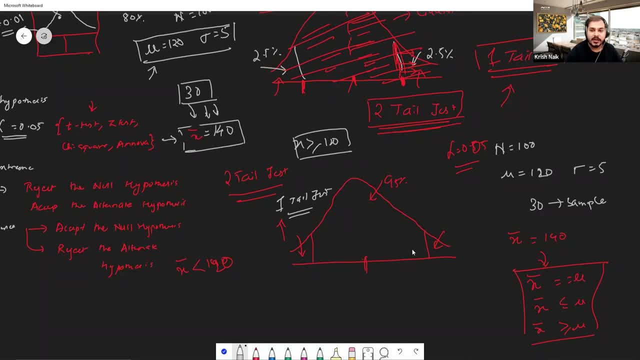 what will it be? two tail or one tail, if you want to just check equality? if i want to just check equality, it will become a two tail test, because this x bar can be less than mean. it can also be greater than me, so both the possibilities are there. 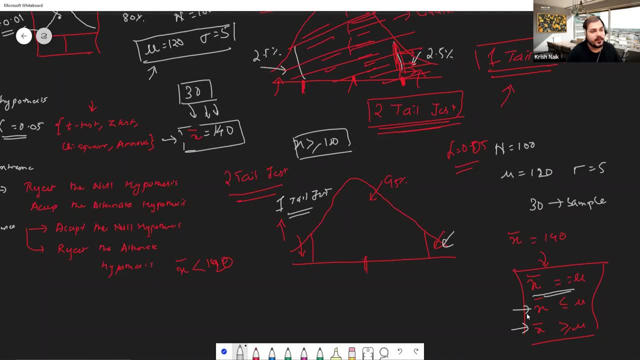 also the five percent. one will be divided in two parts of 2.5 in case of one tail. no, see in one tail if my significance value is point zero. five, okay, if my significance is value is point zero, we will try to divide because, understand this, this distribution is symmetric, right? 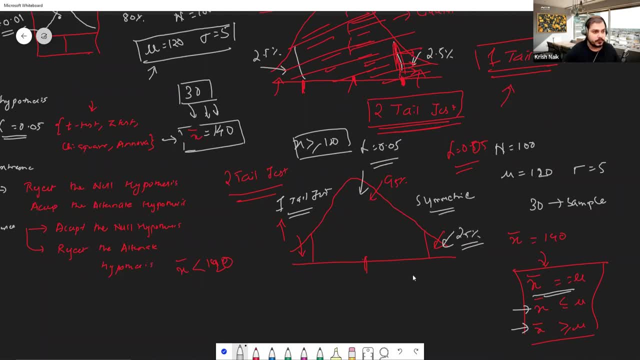 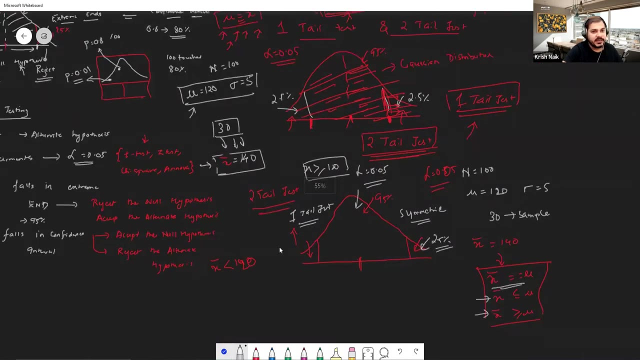 so we just have to take two point five percent, so in one tail test. yeah, we are checking one condition. okay, i'll i'll show you one example. by that you'll be able to understand, okay, okay. So I hope you got some amazing ideas about it. 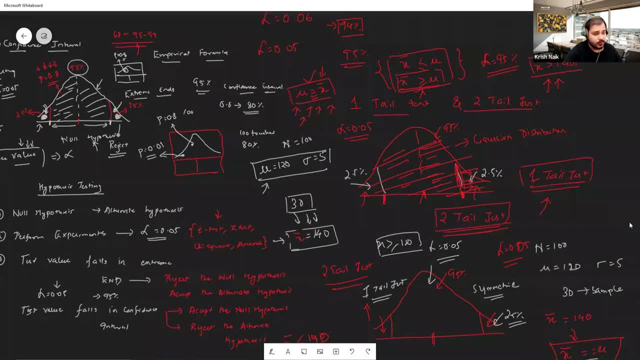 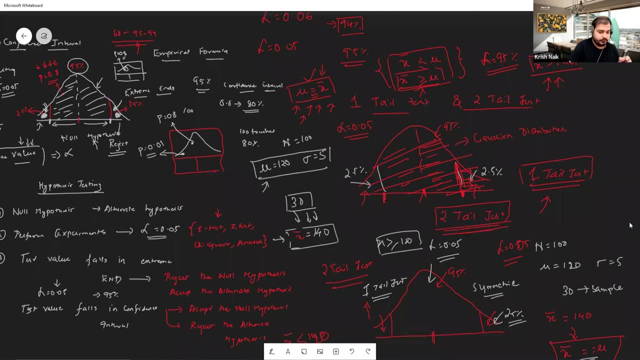 These all are important things You really need to explain in an amazing way to all the guys. OK, OK, OK, nice, Now can I get a quick yes, if you have understood, All good everyone. I think you never saw this kind of explanation right. 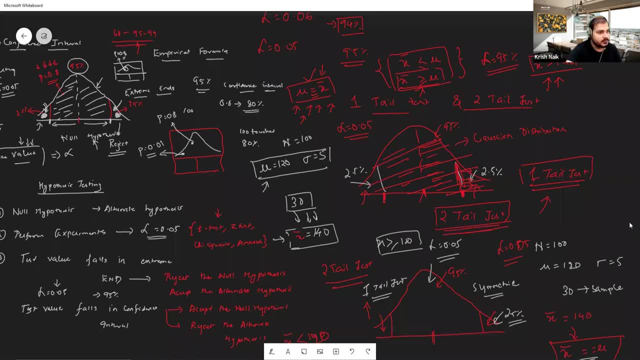 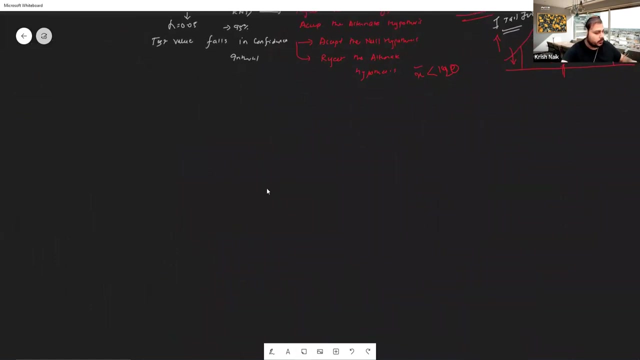 This deep and extreme right For the people who already knew. are your thoughts changing now with respect to the things that we are understanding from here? Yeah, OK, Let's solve a problem Now, the first problem that we usually solve. 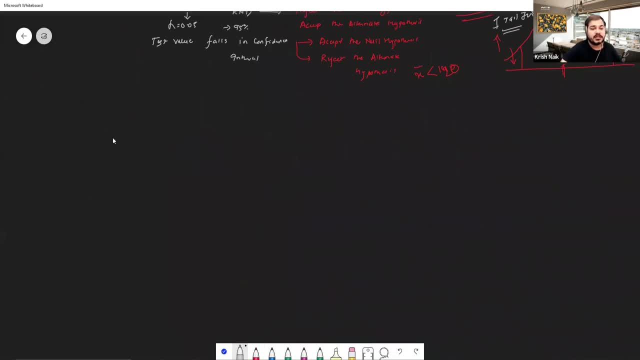 OK, now I did not make you understand. How does a hypothesis testing actually work? So guys understand, always there will be a population. First of all, let me write it down. Suppose there will be a population with some info. OK, with some info. 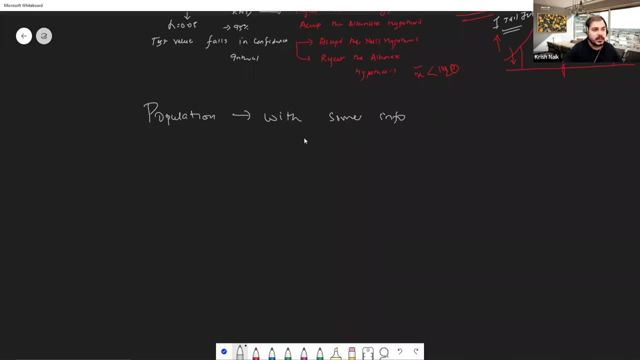 Info basically means standard deviation, Probably mean something, something, something. OK, Then what we do, we take And obviously remember, guys, Can I say, can I just, if I take this particular example, can I say this particular example? 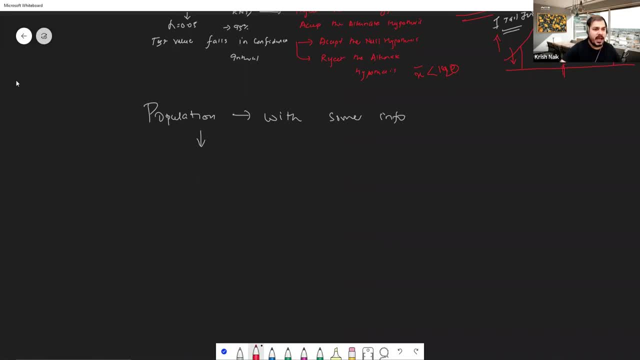 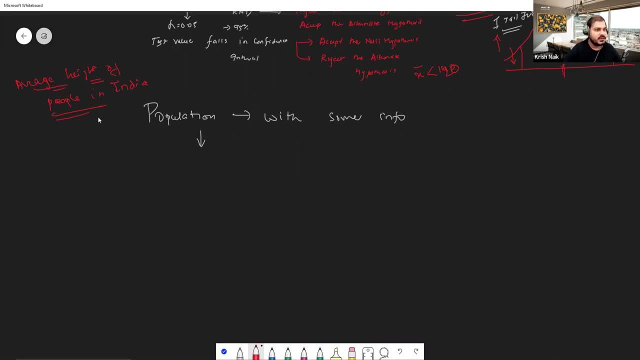 height of people in India. Can I measure this, guys? No right, It is not possible. There are 7 billion people. How many people are there in India? I cannot go and ask each and every person, right? So what happens is that we cannot perform this kind of experiments. 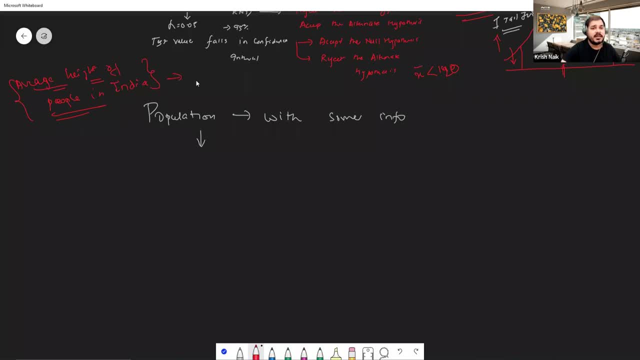 but we can definitely perform experiments by sampling. I can take samples and probably come to some conclusion. Similarly with respect to population, with some info. what we do is that we always try to take some sample and then we perform some experiments. We perform. 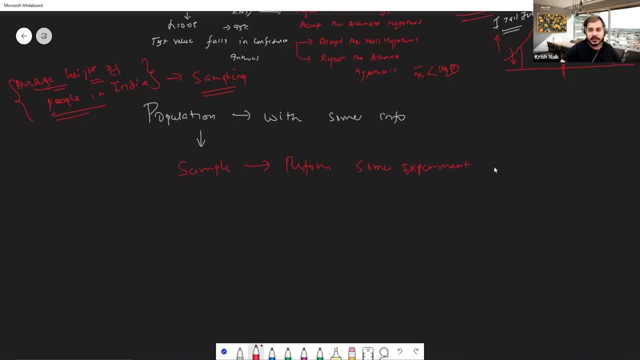 some experiments. Experiments can be any statistical testings. I'll talk about different, different statistical testings. When we perform some statistical testings, from this particular statistical testings we come with some conclusions on about the population. Okay, Some conclusion about the population, And this is the entire. 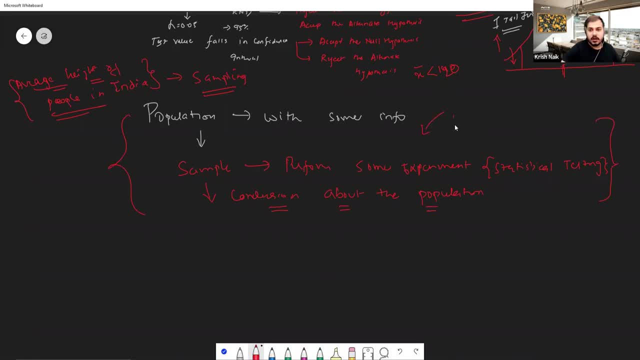 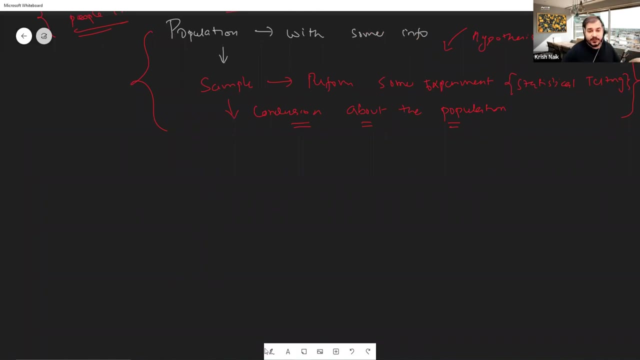 hypothesis testing. We usually do. This is called as hypothesis testing. Okay, Understand this thing. What is exactly hypothesis testing? Okay, Now let's take an example, guys. Okay, What are different types of statistical testings? are there? Please write it down, everyone. So statistical testings. 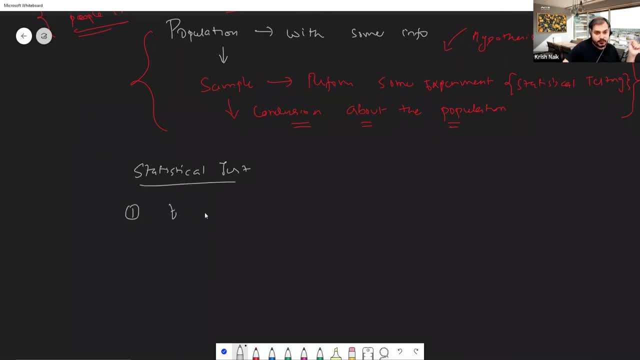 The first statistical testing I would like to say is something called as t-test. Okay, T-test is nothing but comparison of mean. Second one is something called as z-test. This is nothing, but this is also used for comparison of mean Here, standard deviation. 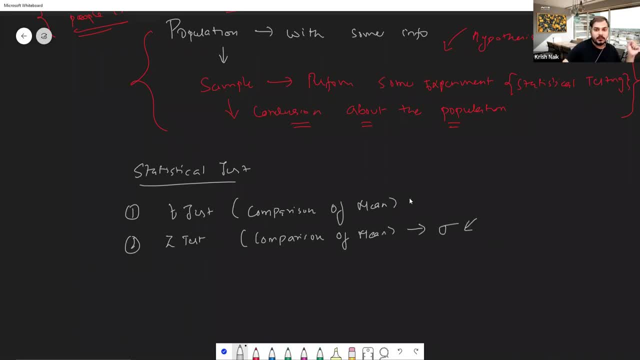 is given, Population standard deviation is given. Okay, Here, sample standard deviation is given, Sample standard deviation. Okay, Here, sample standard deviation is given, Sample standard deviation. okay, here, population standard deviation, standard sample standard deviation is given. if i go to the third one, the third technique that i really want to talk about is anova test. 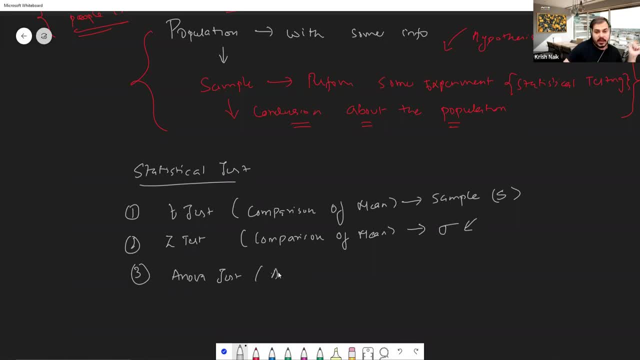 in anova test we do a analysis of variance, whether the variance is same or not. the fourth one is something called an f test. here also we do analysis of variance. sorry, we do comparison of variance here. basically we do comparison of variance, okay. the fifth one that i really want to talk about is something called a chi square. 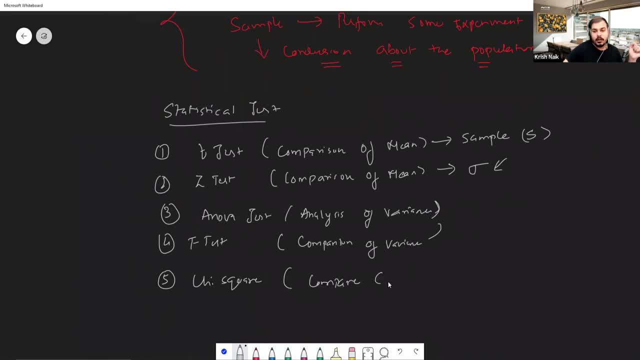 here we can actually compare categorical variables. okay, so we will try to see some of the techniques in this and uh, yes, i have also uploaded videos on this with respect to practical implementation, and okay. so let's start the first one, and the first test that we are actually going to do is something called as one sample. 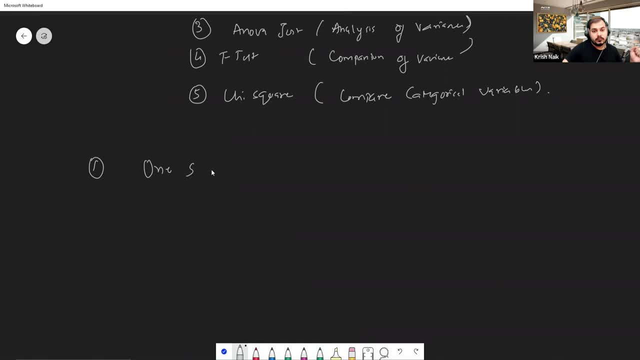 z test. so hi, it's me anna. okay, so this is the first one with that we are going to do with respect to the statistical thing, okay, okay. so size of the sample size also matters in t-test and z-test, right n is greater. yeah, i'll talk about it, okay. 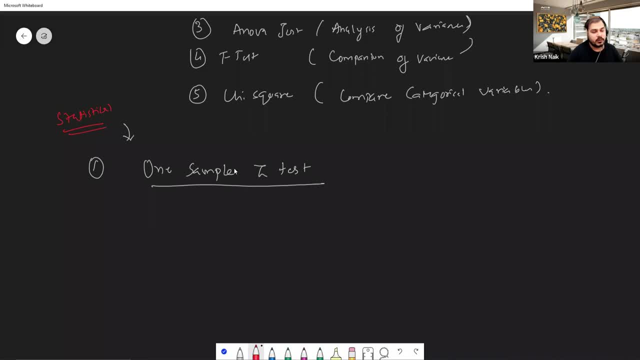 which? which one you want? uh, at least 30. only z test. you only want more than 30.. In t test it is not required. So there are a lot of many things that we will be discussing. OK, I'll talk about that when we discuss. 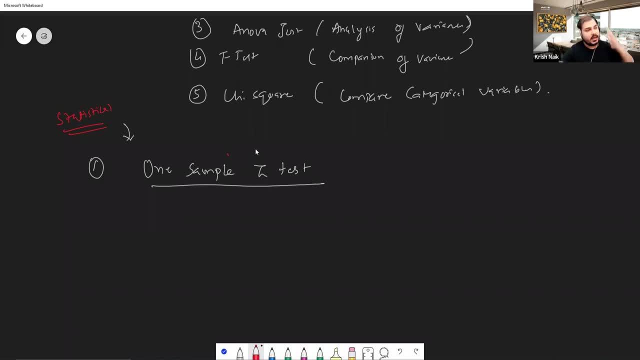 the complete testing itself. But till here, everybody's cool enough. Everybody's cool enough. I hope you're having the positive feeling that you can understand all these things. Yeah, OK, perfect, OK, now I have a problem statement. Everybody write down the problem statement, guys. 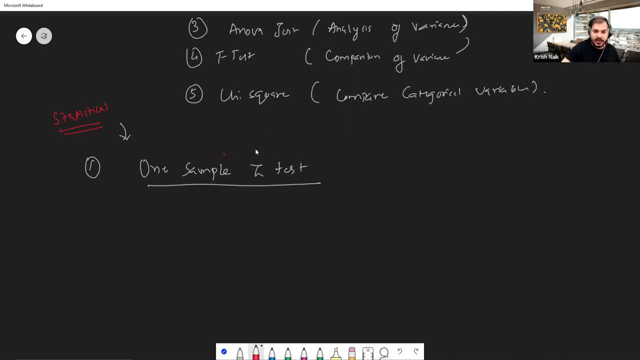 Everybody write down the problem statement. OK, So I'm just going to write it over here for you. OK. So in a population, everybody write it down. In a population, The average IQ mu, average IQ. within a population, the average IQ mu is equal to 100,. 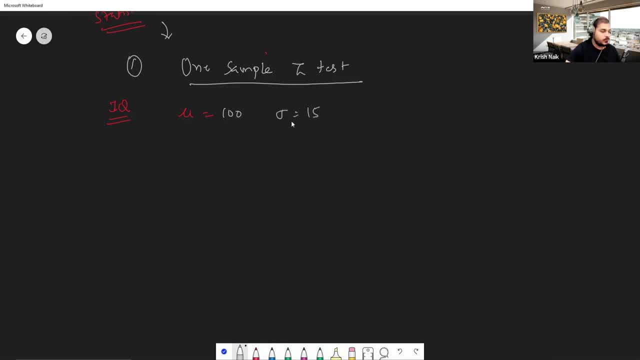 with a standard deviation as 15,. OK, In a population the average IQ is 100, and standard deviation is equal to 15.. So basically, the average IQ mu is equal to 15.. Then the doctor tested a new medication to find out whether it increases the IQ or decreases the IQ. 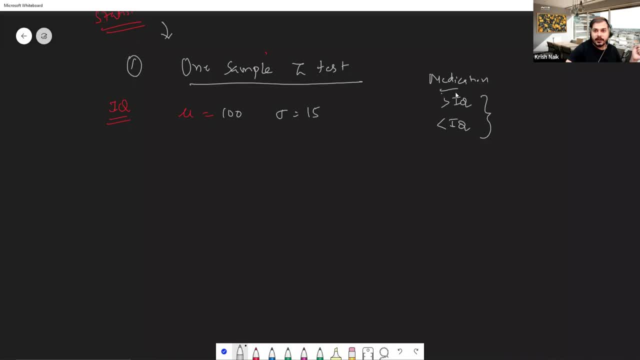 This is basically a medication that has been provided to the population. OK, So the doctor tests a new medication, whether it increases or decreases the IQ, the IQ Then, after doing the medication, probably after one month, after one month sample of. 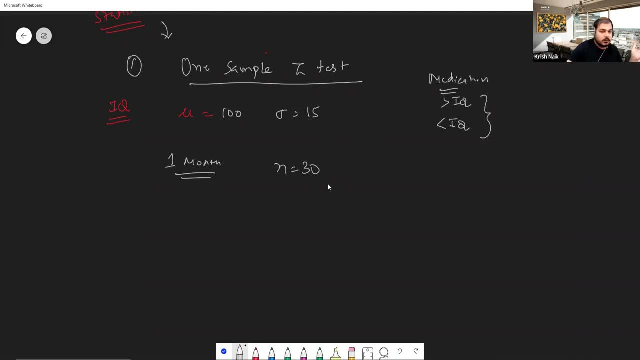 30 people, 30 people or 30 participants- okay, sample of 30 participants were taken after the medication after one month, guys right, And this 30 participants had a mean of sorry, this mean I can write it as X bar had a mean of X bar 140.. So our question is: did. 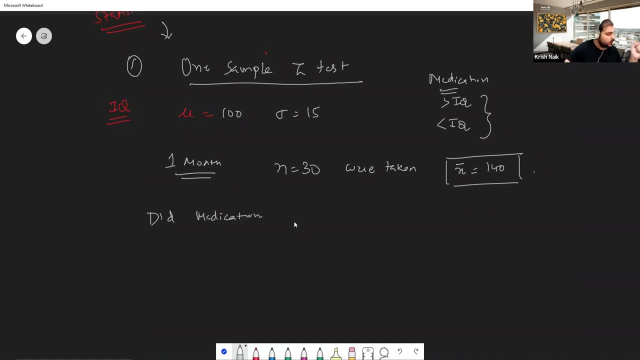 medication affect intelligence. Everybody understood the question Here. your significance value is 0.0.. This is also given- Again- I'm repeating the question- In a population. in a population, the average IQ which is given by this mean is nothing but 100.. With a standard IQ of 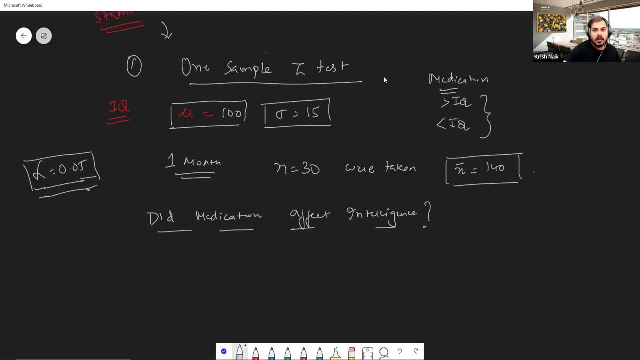 100,. you have a standard deviation of 15,. okay, Doctors tried a medication to that particular population to see whether it increases the IQ or decreases the IQ. okay, Increases or decreases the IQ, okay, Okay. First of all, you have to define the null and the alternate. 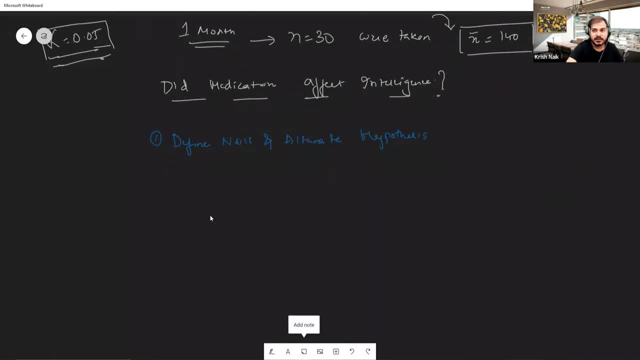 hypothesis. Can anybody tell me what is the null hypothesis? Null hypothesis is usually given by H0.. Can anybody determine the sources of mu positive or non-positive mu situation? Here the null hypothesis see, did the medication affect intelligence? okay, So here my null. 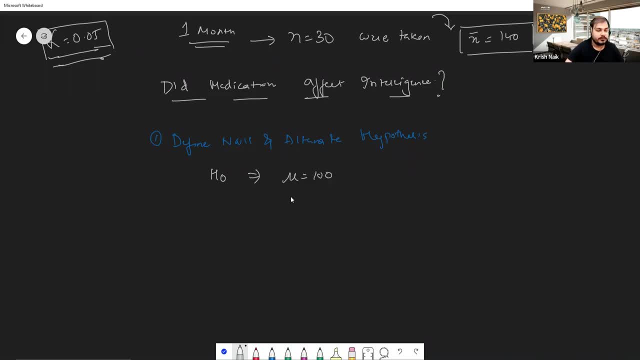 hypothesis will be: mean is equal to 100,. okay, I hope everybody is able to understand right. My null hypothesis is: mean is equal to 100, because what we are testing- whether my mean is changing or not- my initial population mean was 100, right, So my null hypothesis. 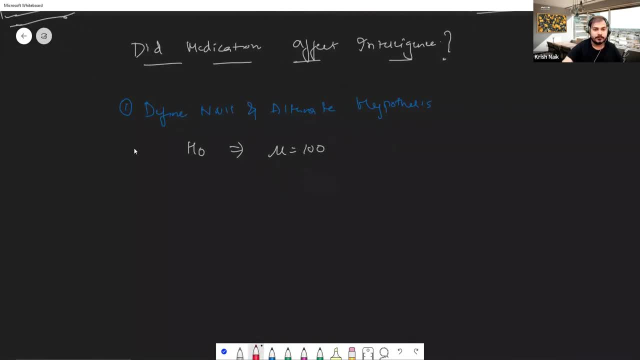 will be mu equal to 100.. mu is equal to 100. So let me write it down. So this is basically my null hypothesis. Okay, Divya, how can X bar be 100?? See, you are not understanding the question. What did? 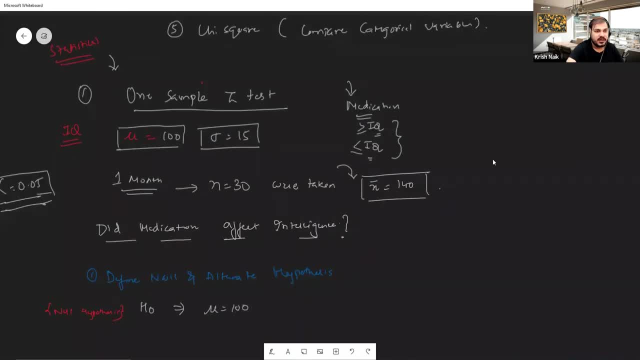 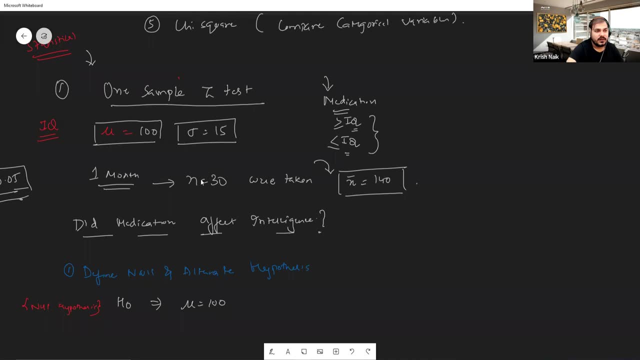 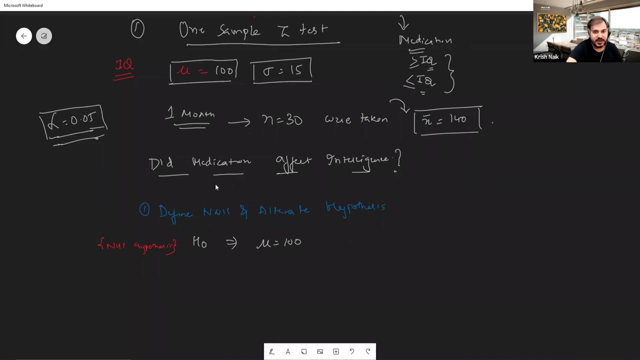 I write over here. The average IQ is 100, right, Did I say 140?? X bar is 140, no, When we say null hypothesis- yes, I am here, I am writing right- Your null hypothesis is: mean is equal to 100.. We need to check, right, whether the medication affect the intelligence. 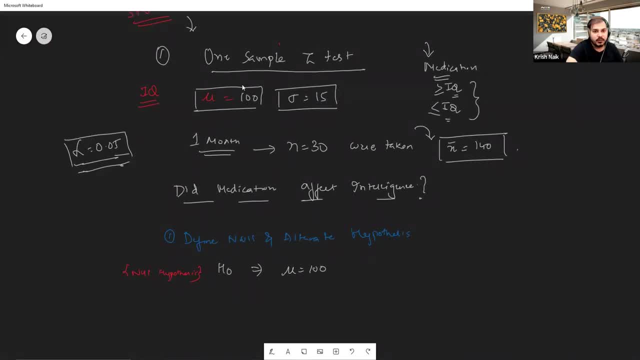 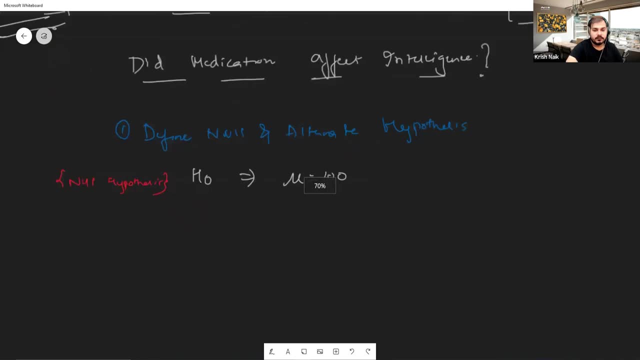 or not. That basically means whether the IQ is 100 or not, right? So in the null hypothesis we will write: mu is equal to 100, okay, Okay, Now let us go to the alternate hypothesis. What is alternate hypothesis Mean is not equal to 100. 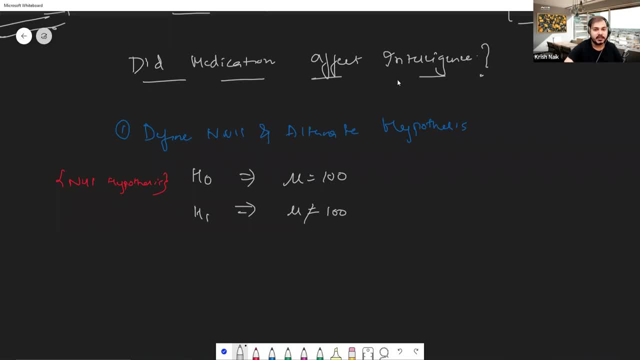 Because we need to check whether the medication affect the intelligence or not. I hope everybody is able to understand what is null and alternate hypothesis. We really need to check whether the mean is equal to 100 or mean is not equal to 100. Okay, Clear, Everybody clear, Okay. 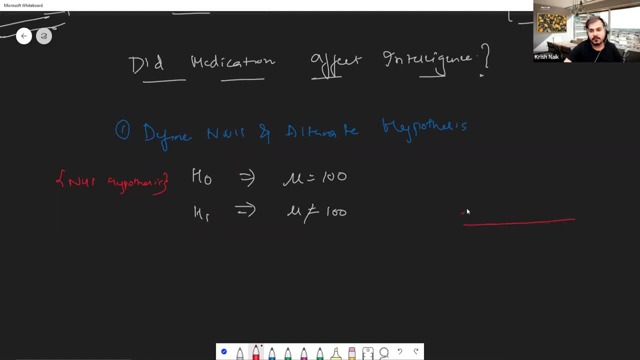 Now tell me whether this is one-tailed test or two-tailed test. It is a two-tailed test. What is the Alpha value? 0.05.. So what should be my confidence interval? 95%. So this will be. 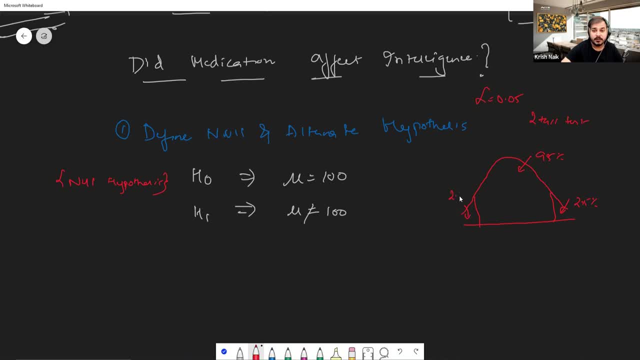 my 2.5, this will be my 2.5.. I will talk about this. why it is important. Okay, Why it is important? Okay, perfect, Now, this is my first step. Now, this 2.5, this is my first. 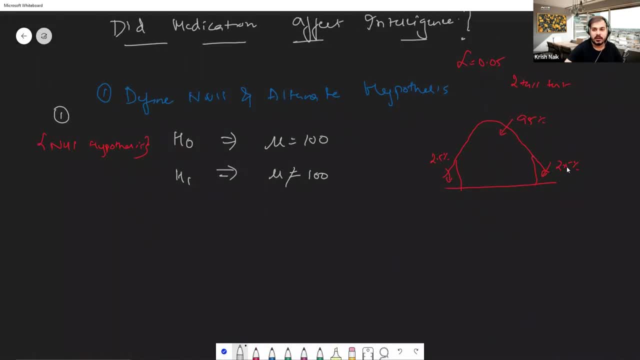 step Now. this 2.5 can be written as- sorry, it should not be written, as it can be written as like this: 0.025, 0.025. Okay, And this will become 2.5%. Okay, Now, this is my first. 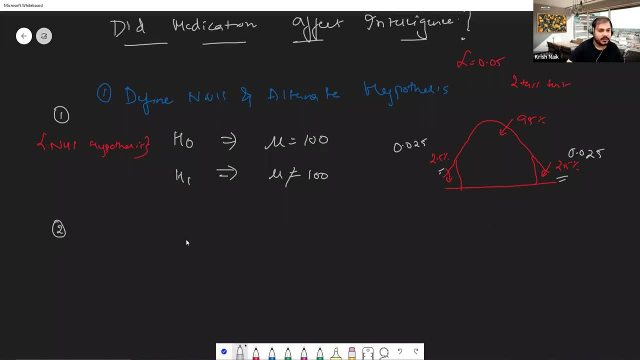 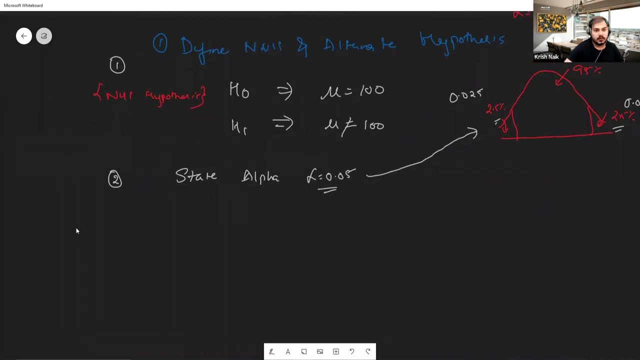 step. What is my second step? What do we do in the second step? State the alpha that we have defined. What is alpha 0.05.. And because of that, we know that it is a two-tailed test. Perfect. Now come to the third step. What is my third step? Okay, What is my third step? 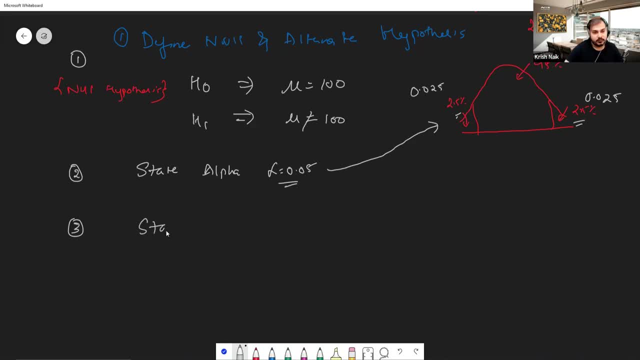 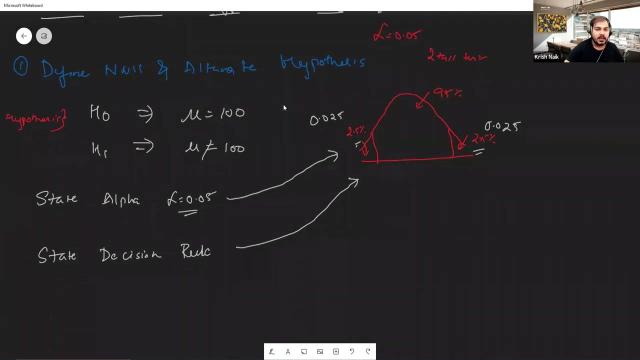 Now my third step is basically state decision rule. State the decision rule. Now, this is very, very much important, guys. Okay, What is the decision rule? Again, this is related to this particular graph only. Okay, Now, just imagine I told you that, in order to check this, whatever experiment that I 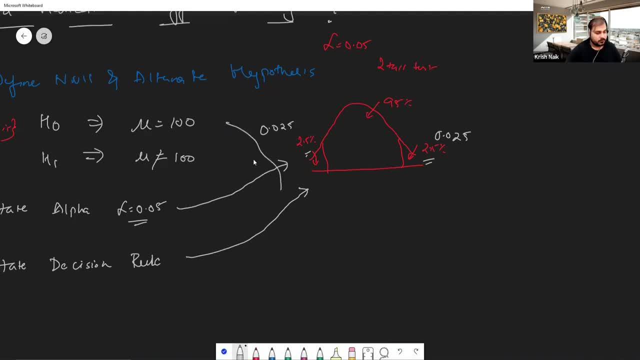 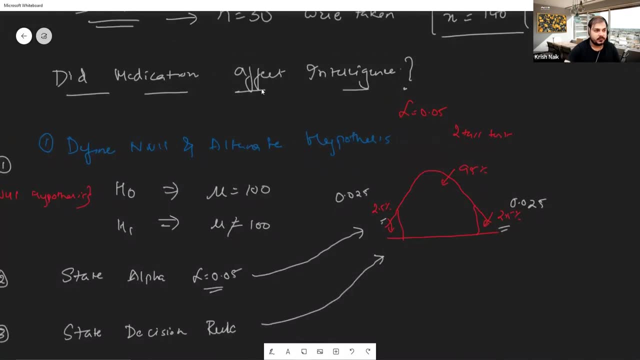 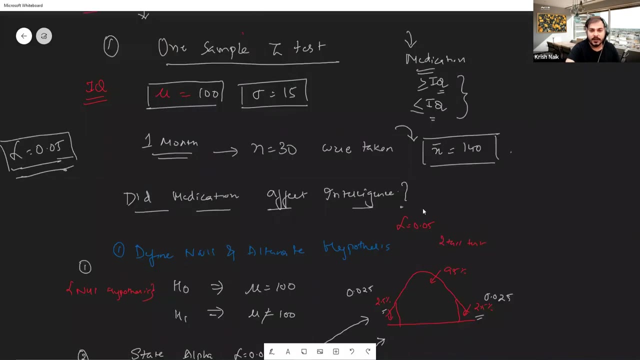 will be performing. here the experiment name is something called as. here the experiment name is something called as what it is: One sample Z test Right. One sample Z test Right. One sample Z test. So, according to the experiment we need to perform, we need to provide the 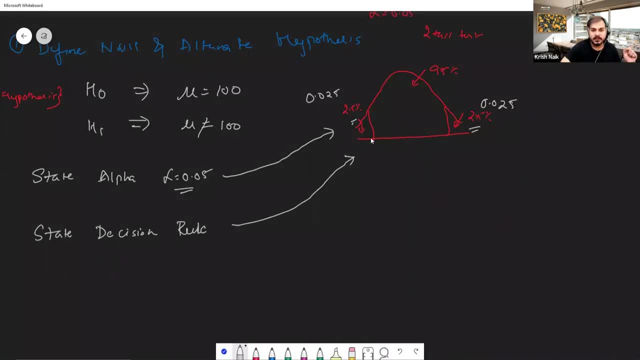 decision rule. Decision rule basically means we need to provide the decision rule Decision. what will be this value to this value? what is this range? we need to find out. okay, we need to find out now. everybody knows this. this region is nothing but 0.025. yes, this region is also 0.025. 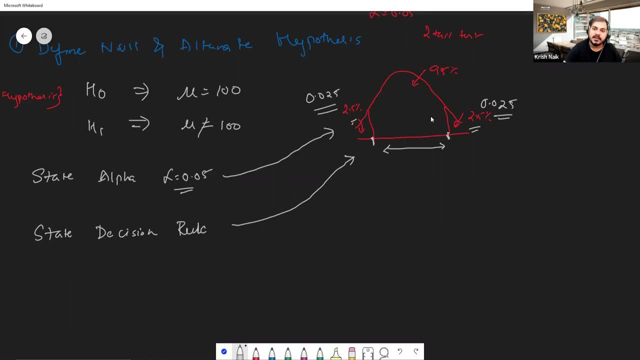 okay, if i consider the entire region, how much is the entire region, guys? full entire region. can i consider it as one? okay, entire region. can i consider it as one? yes, now just imagine, if i subtract 1 by 0.025, what will be this particular region. 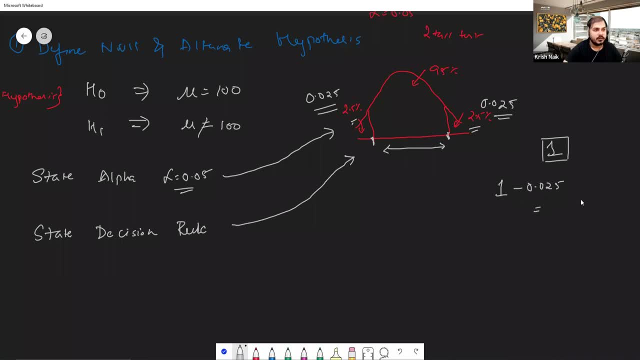 what will be this particular region? 1 minus 0.025 is nothing but 0.975. do you agree with me? so this is 0.975. This basically means that if I take this 0.025, can I consider this will be my entire region? 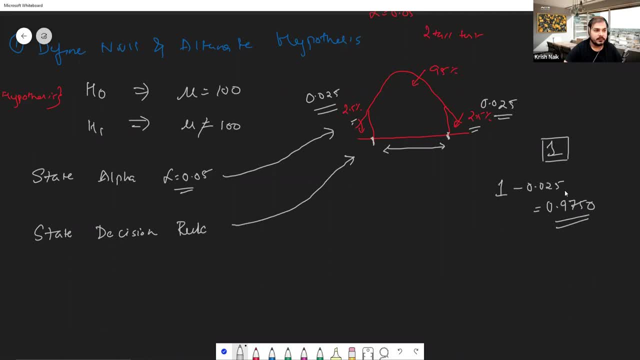 if I just subtract 1 minus 0.025?? Sorry, just let me do the subtraction Calculator: 1 minus 0.025.. So it is nothing but 0.975.. I was right, people are confusing me- 0.975.. 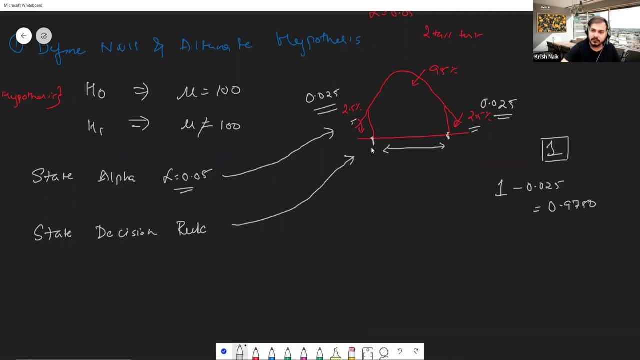 So if I try to do this, this is basically my entire region like this. right, I really want the values between these two. So what will happen, See, if I try to find out what will be this particular value? suppose this will be some. 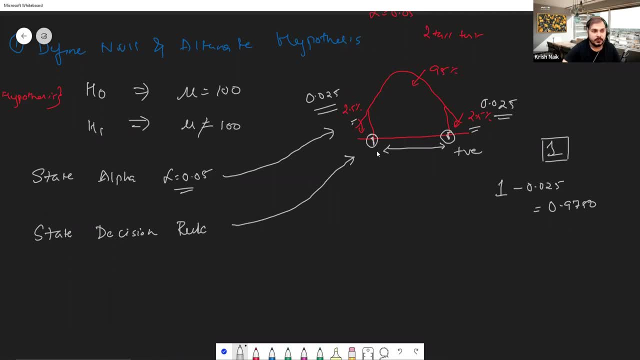 positive value, then what will be this value? It will be the same negative value. Do you agree with me or not? Yes or no? Tell me, guys, Because this is symmetrical right? Whatever things are there in the right-hand side, the same thing will be there in the 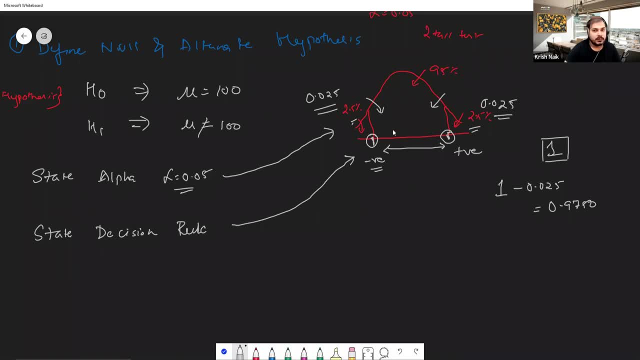 left-hand side, right. And what is Z-score guys? What is Z-score? Why it is basically used? It is basically used to find out how many standard deviation is away from the mean. Do you agree with me? How many? 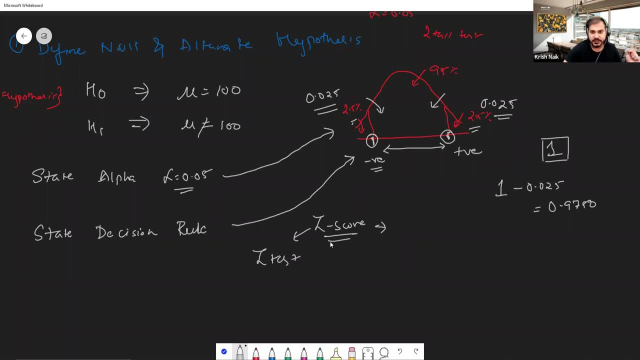 And that is true. It is the same related to Z-test. In Z-test, we will try to find out. what is this specific range? So, in order to find out, let's go to this right-hand side, In this right-hand side. if I really want to find out, I'll just subtract this one area. 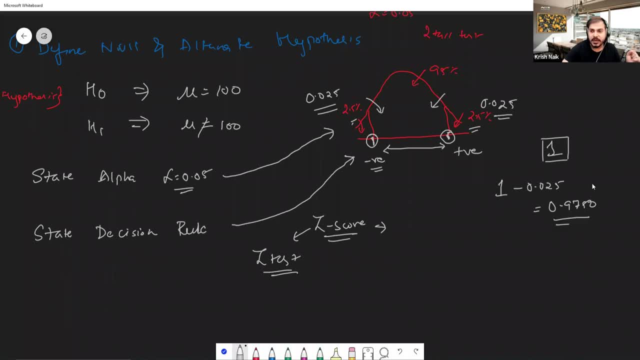 by 0.025.. I really need to find out the area under the curve of 0.9750.. Now, in order to find this, I will be using something called a Z-table. So let me just show you what is Z-table. 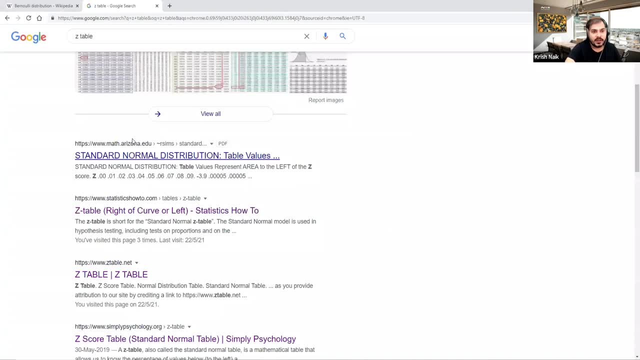 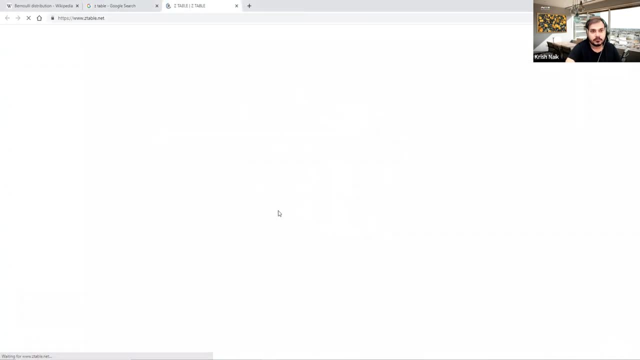 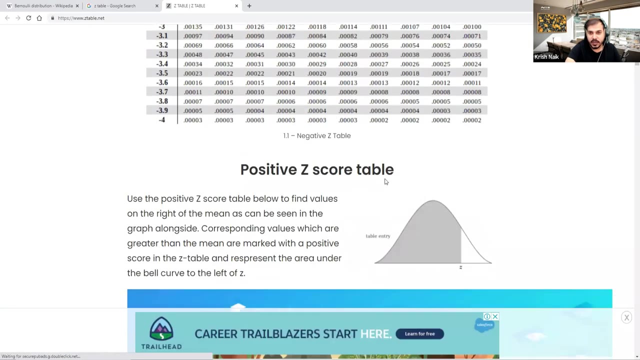 So let me just search for Z-table. So if I go and see Z-table, Z-table, just go and see over here where does 0.9750 fall. See, if I go down, where does 0.9750, it is falling somewhere here, right? 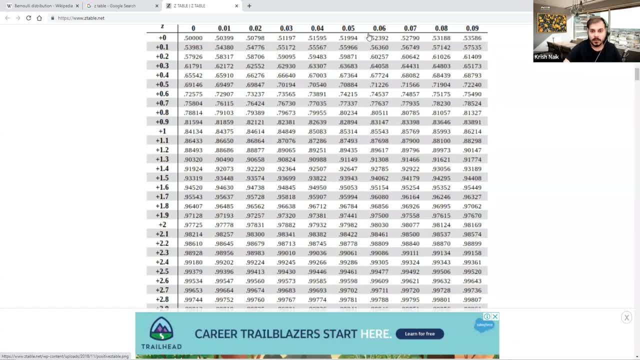 See over here. Do you see this? Do you see this 0.9750? Area under the curve Right? So what is this particular value? This value is nothing but 1.9.. And if I go on the top over here, it is nothing but 0.06.. 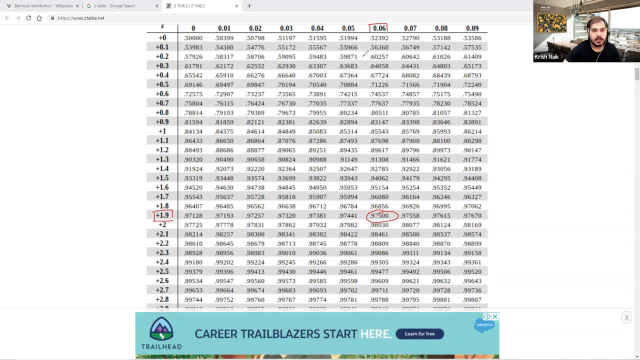 Do you agree with me? So the total value for this particular area under the curve will be 1.96.. Okay, 1.96.. Now I have found out in the right-hand side what should be my value: 1.96.. 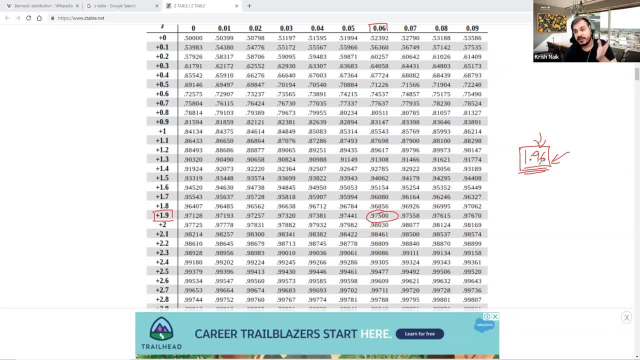 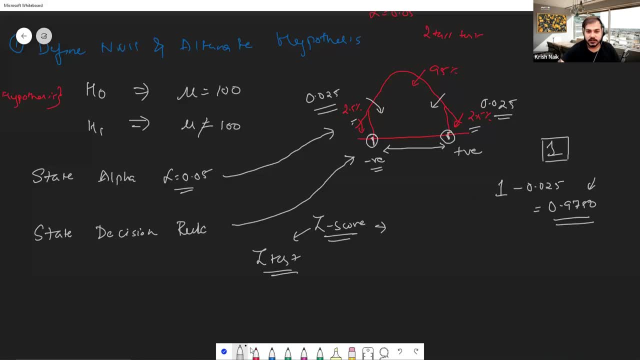 So this is nothing, but it is 1.96 times 0.9750.. Okay, That is my standard deviation away from the wind. Okay, So now I will go over here. I will go and take out this particular range. This range is nothing but plus 1.96.. 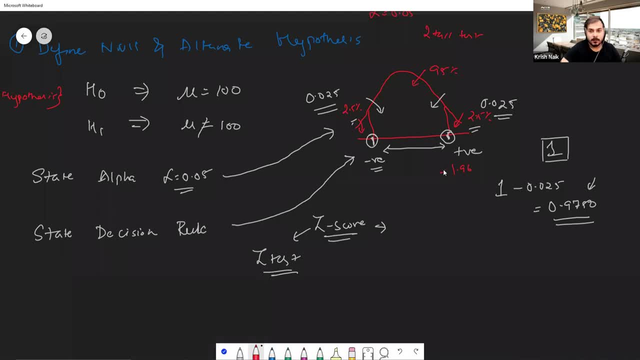 So what will be this particular value? If this is plus 1.96,, what will be this particular value? What will be this particular value? Come on guys, tell me Minus 1.96.. Very simple Now. whatever experiment I am performing, it should be ranging between these two values. 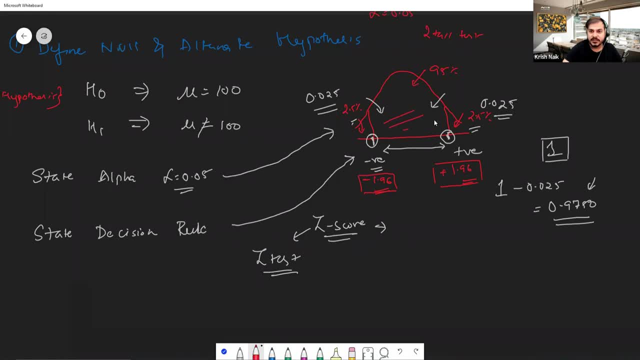 If it ranges between these two values, that basically means it will fall inside this 95% confidence interval. Then we can accept the null hypothesis and we can reject the alternate hypothesis. But what if it falls less than 1.96 or greater than or equal to 1.96? Then what we can. 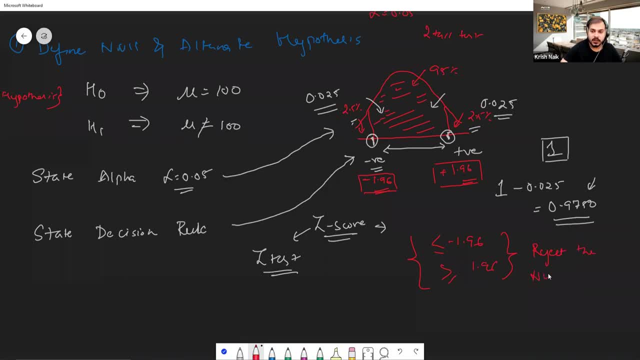 do? We can reject the null hypothesis and accept the alternate. Okay, Guys, is it clear? everyone? So this is my decision rule. My decision rule says that I need to: basically whichever experiment I am performing, it should be falling between minus 1.96. 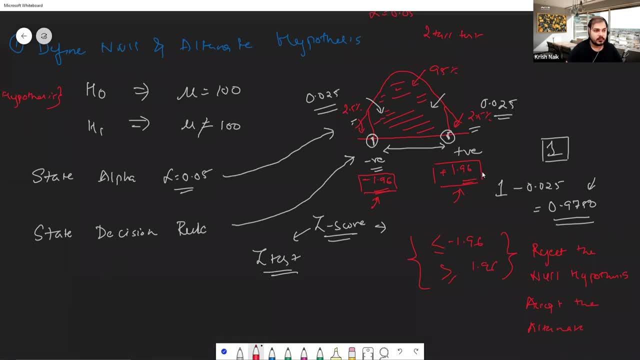 to plus 1.96.. Okay, Understand guys, why we are doing this? Because we don't have much information, right. We just have the information: How much percentage? What is the alpha value? This is the importance of alpha value. Okay, This is the importance of alpha value. 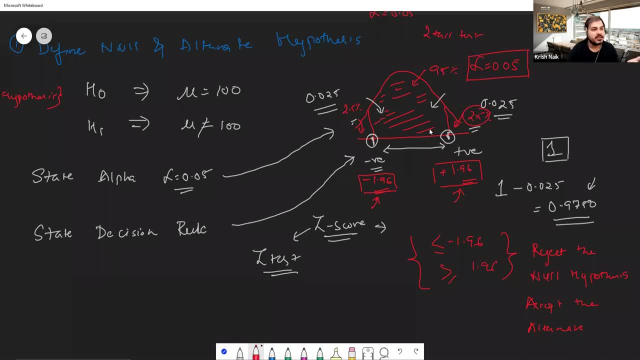 How you are going to compute the Z-score divya. You don't have any information. No, You just have this alpha value information If you want to compute the Z-score divya. you don't have any information, No, You just have this alpha value. 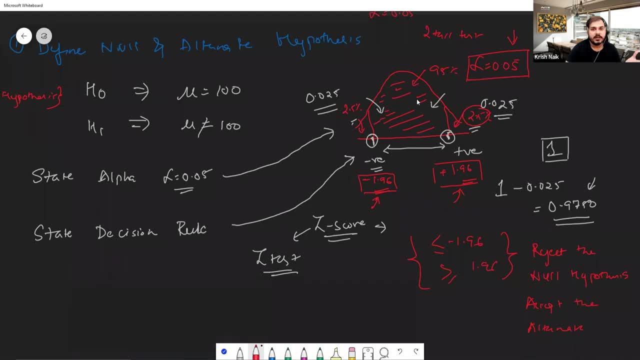 information. If you want to compute the Z-score, how you will be doing it, Trust me. That is not X bar minus mean, It is X of I. You require data points. divya, Did I say? Okay, guys, what is Z-score formula? Come on, You are just again missing up the entire thing. You are messing up. X bar minus mean will not be there. X of I minus mean, divided by standard deviation, will be there. You don't know the data points, right? 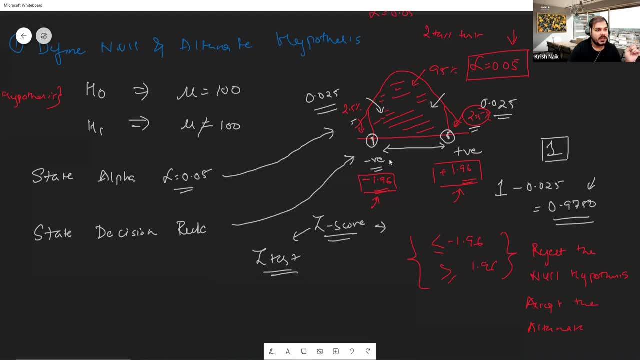 Sir, why the equal to? Are you talking about this, Jay? Are you talking about this, Jay? Okay, sorry, Let me do one thing. Let me make it less than or equal. Okay, I just wrote in the flow. 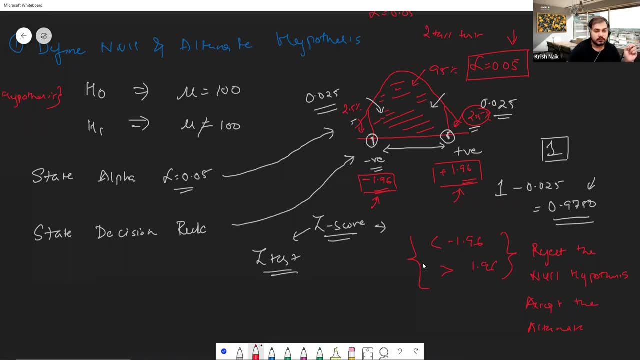 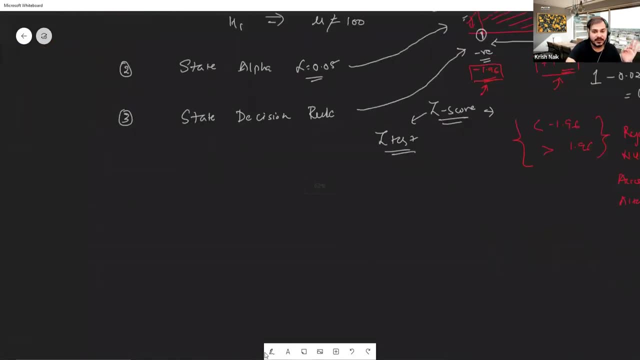 Okay, Is it fine now? Okay, Now let's start performing the experiment. Now, how does the experiment? And see, guys, for this kind of experiment there are some kind of fixed formula, But always understand the process. What did you do First? 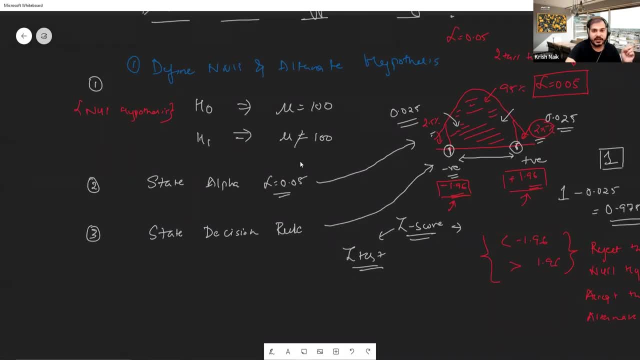 process, you define the null and the alternate hypothesis. Second, you stated the alpha value. You understood. okay, this is a two-tail test. Then you found out the decision rule. In decision rule, you found out that it should be ranging. 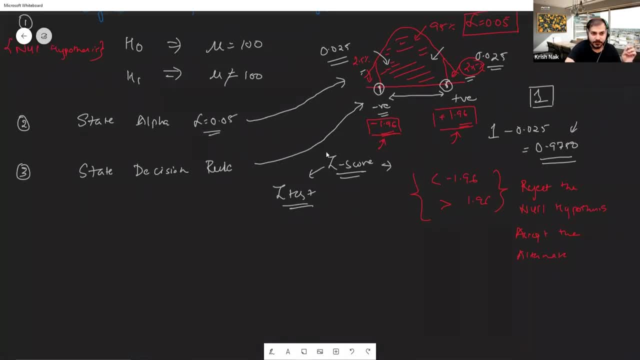 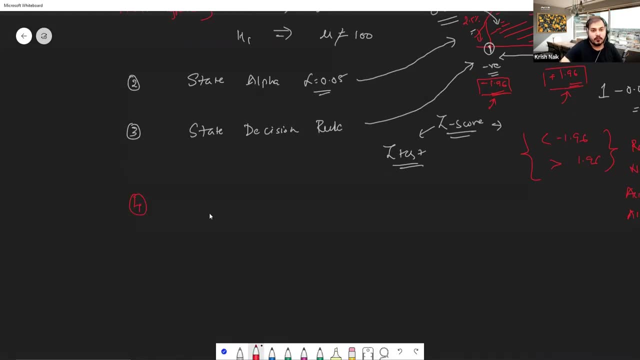 between minus 1.96 to plus 1.96.. Okay, Now the fourth step. The fourth step is nothing, but It is a very important step. again, Let's compute the test statistics. Fourth step: Let's compute the z test. let's apply: z test is basically given by a formula, guys. 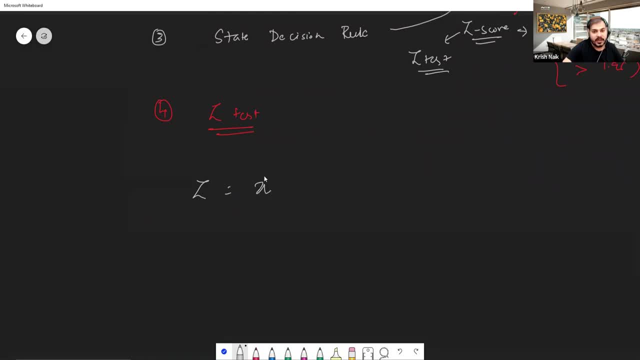 z is equal to x bar minus mu. okay, this is z test formula, not z score. okay, always understand. this is z test to find out what value it will come divided by root n. okay, what is this x bar? x bar is nothing but sample mean. always remember this formula, guys. again, i'm not going to derive this. 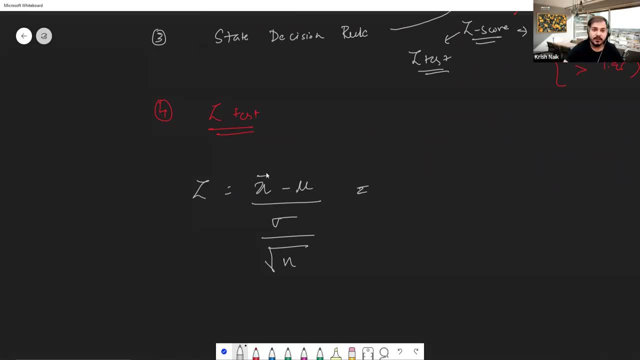 particular formula but to in order to find out that area under the curve. we basically apply this particular formula in z test. okay, x bar is what, guys? 140 minus 100 divided by 15 root of 30. if i go and compute this, guys, it will be nothing but 40 divided by 2.74, it is nothing but 14.60. 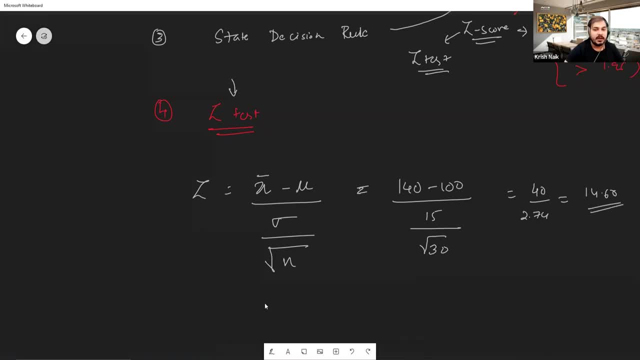 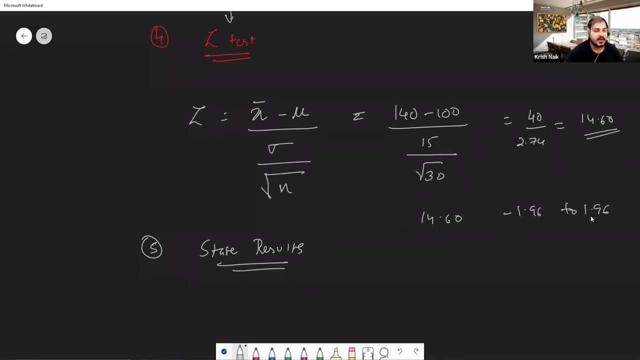 now, guys, you have got 14.60. now tell me, tell me which. the last step, okay, the fifth step, after computing the z statistics. here we will now state the results. now tell me, guys, whether 14.60 falls in the range of 1.96, 2 plus 1.96. does this fall in this range? 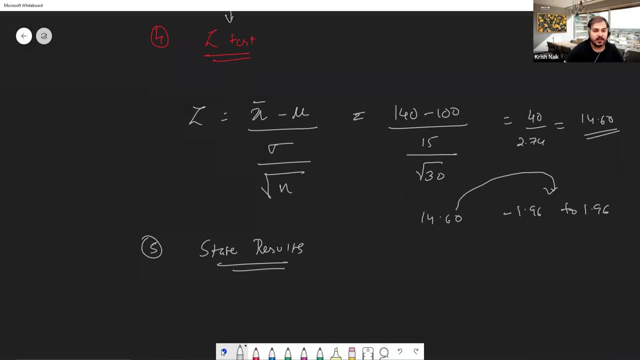 does this fall in this range? no, so now tell me what should be your alternate: whether you should reject the null hypothesis or accept the null hypothesis. so, since my value is 14.60, it does not fall between. it does not fall between minus 1.96 to 0.96, though. so what we do? we reject the null hypothesis. 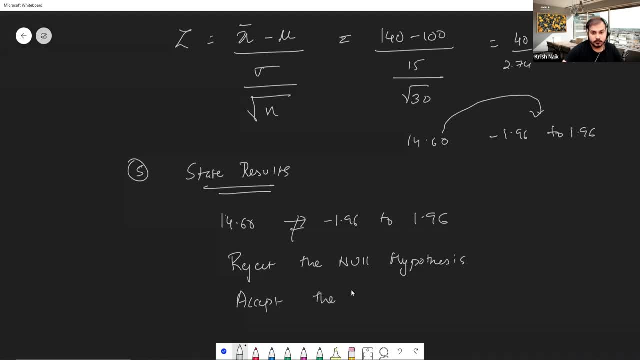 and we accept the. so this is my entire result. amazing, right. it means definitely there is a change in iq. there is a change in iq. so this is my entire result. amazing right. it means definitely there is a change in iq. so this is my entire result. amazing right. 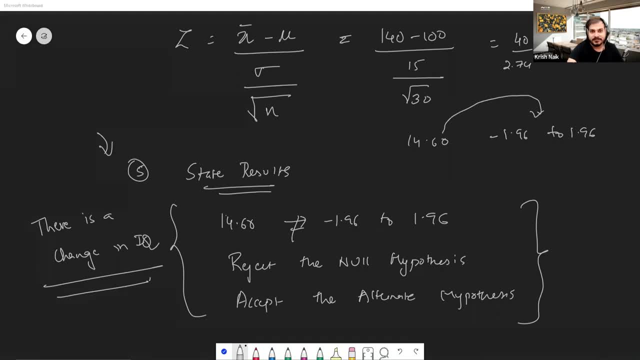 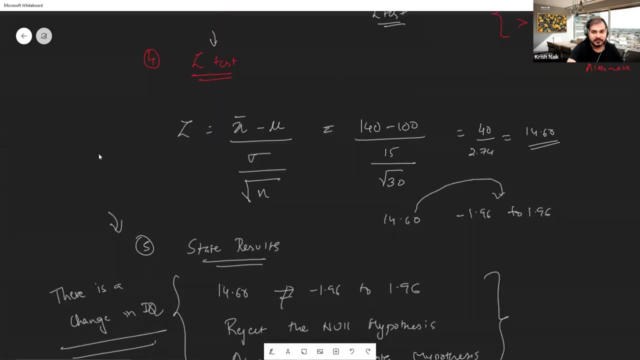 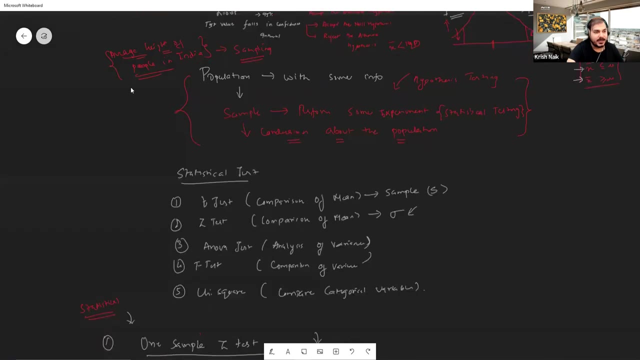 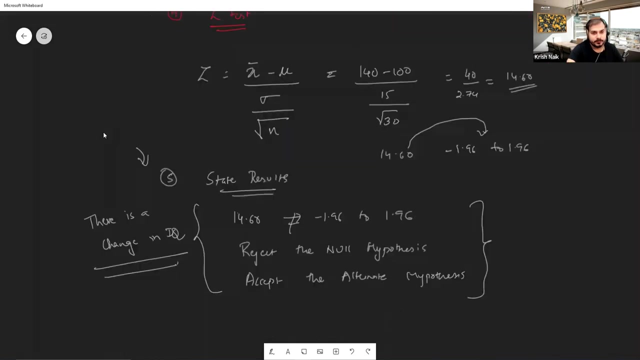 so how do you write to rate this particular explanation? i think you have seen many videos, right, guys? did you understand like this anywhere? did you understand something like this anywhere? did you see this kind of explanation before, guys, again, this is not the knowledge from college you know, or school. 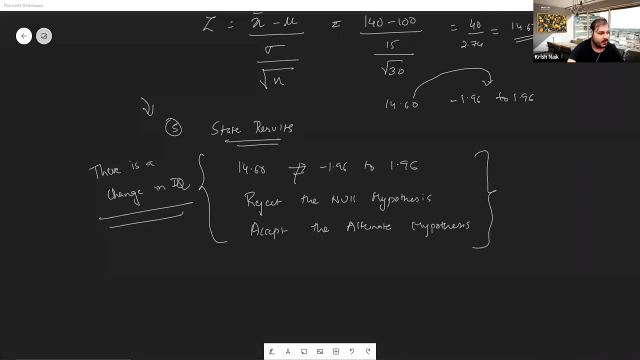 okay, this is not knowledge from college or school, right? okay, now try to perform the same experiment here. now try to perform the same experiment here. let's take the alpha value as 0.1. now tell me, guys, what will be the answer if i take alpha as 0.1. suppose my new domain person comes and says: instead of taking 0.05, 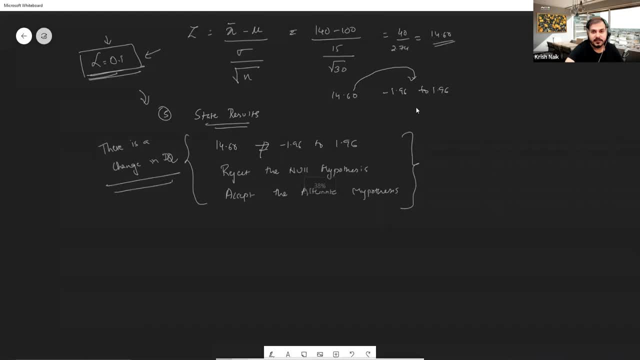 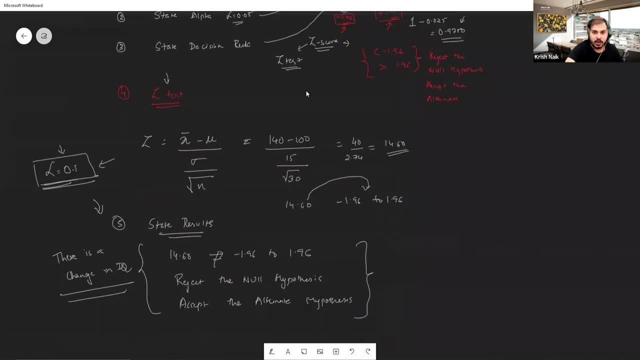 take: alpha is equal to 0.1. now try to do it, guys, from your side and tell me whether we should reject or null alternate hypothesis or accept it. what is this particular value that we will get? first of all, draw this, state the decision rule. what should be the range of this particular? 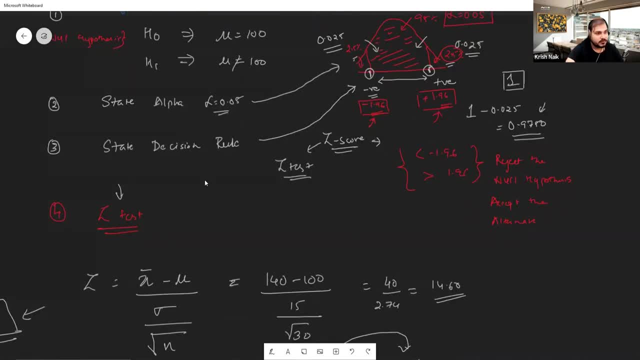 decision tool. it is very, very much simple. now, can you do this, everyone guys? will you do this or not? if your alpha is 0.1, alpha is 0.1. right, if i subtract 1 minus 0.05, what it will come? 1 minus 0.05. 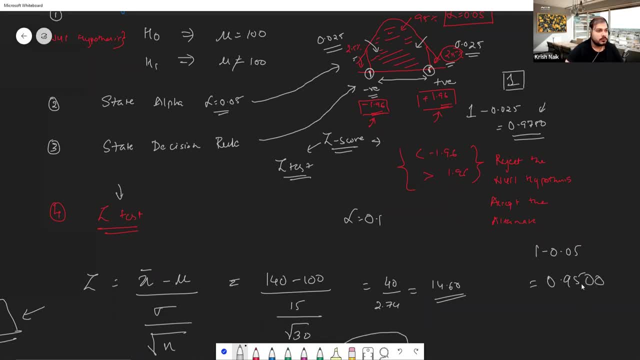 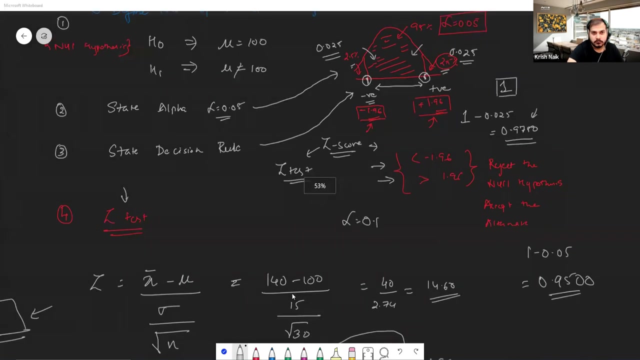 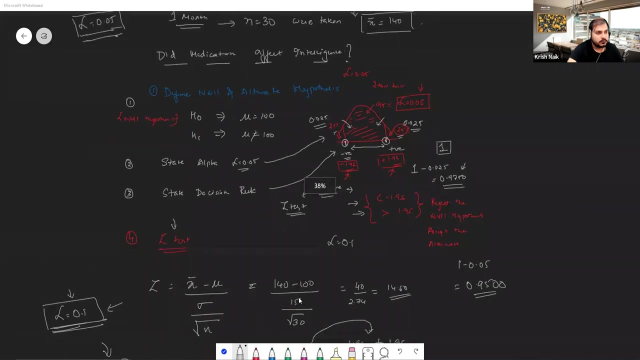 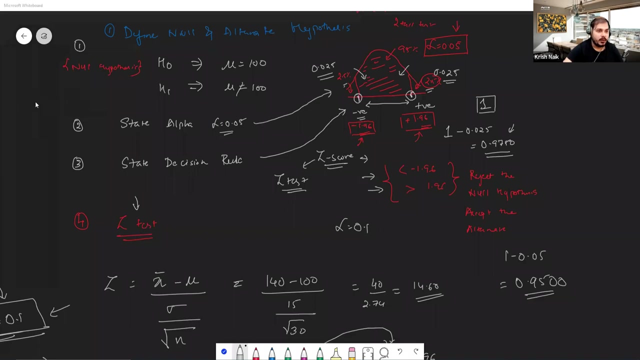 0.95, 0, 0. go and find out what will be this 0.9500, and then here you will be able to get the range of 0.45 When I am taking the alpha value as 0.1. okay, just understand if I am taking. 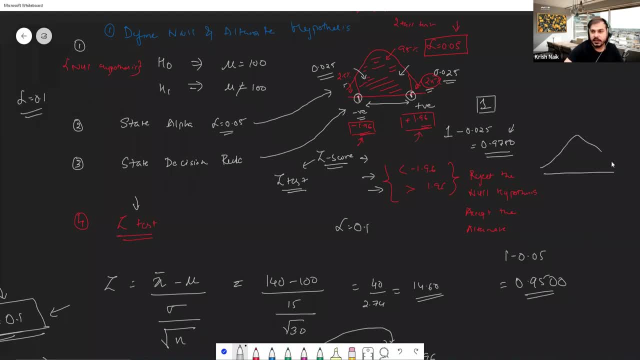 alpha value as 0.1. that basically means I am drawing this kind of thing and this is like 90% percent confidence, right? ninety percent confidence, then five percent will come over here, and five percent will come over here. so manath, try to see this now. did i say 0.01? i'm not. 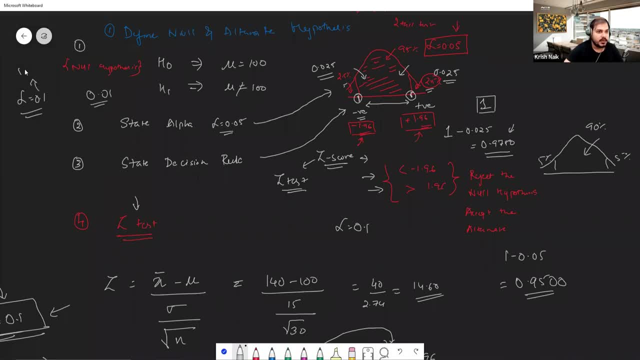 saying 0.01, i'm saying 0.1. this 0.1 is nothing but 10 percent, so the range between it should be 1.65 to 1.65. okay, perfect. again we need to reject the null hypothesis. okay, clear everyone. 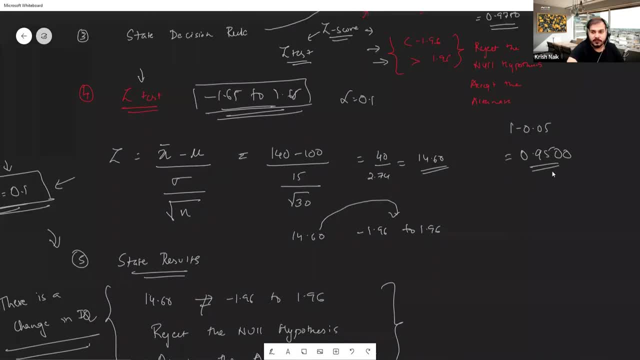 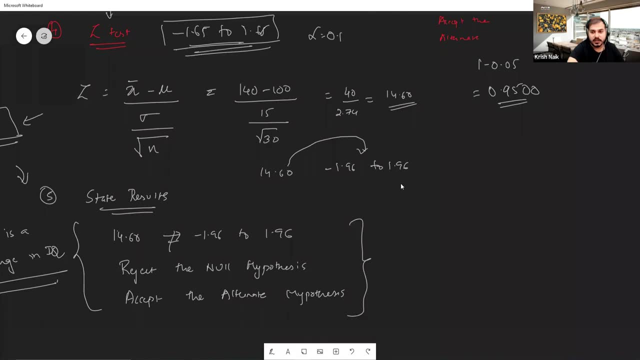 so, guys, whatever computation we did from this z test, okay, we got the value as 14.60. we know 14.60 does not fall between minus minus 1.96 to plus 1.96. so what we do? we reject the null hypothesis and accept the alternate hypothesis. that basically means there is a 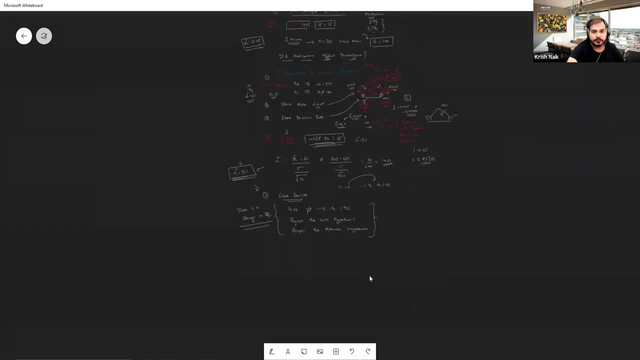 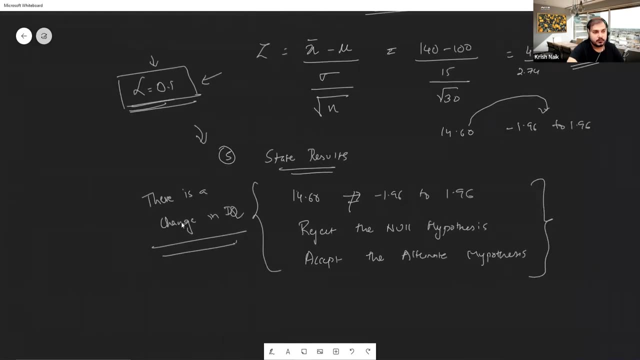 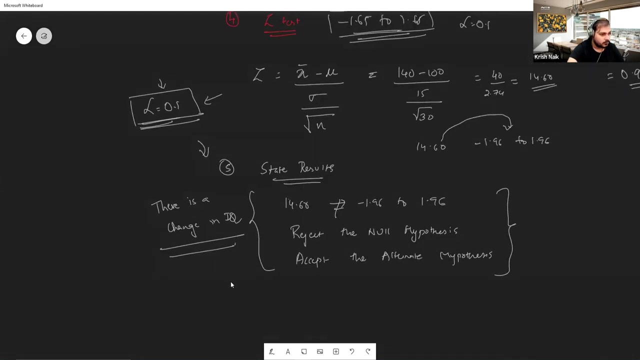 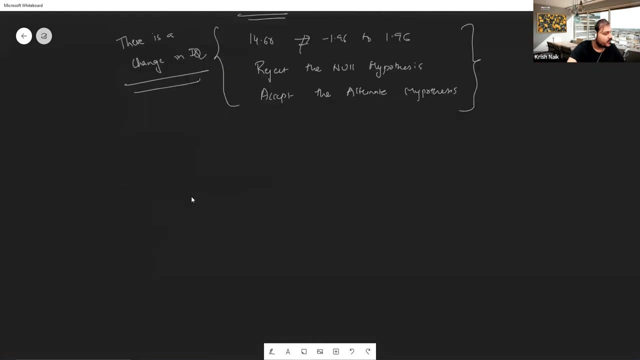 0.65. there is a change in the iq. there is a change in the iq. okay, okay, now let's start the next topic. now we have something called as. this is one kind of test with respect to z test. we also have one test which is called as. 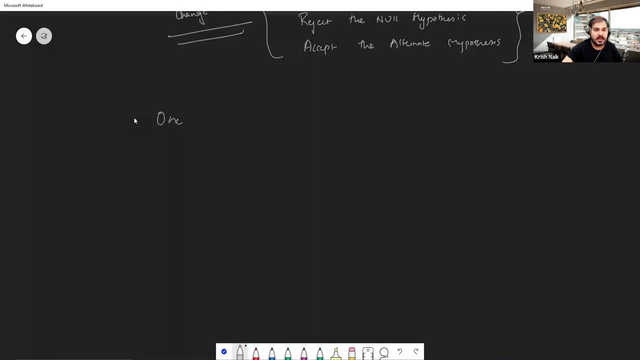 z test, which means z test with proportion. one sample- this is the first one- one sample z test with proportion. one sample z test with proportion or four proportion. okay, shall we start this? okay, Thank you, You got to know. the IQ is changed, but whether it is positive or negative, 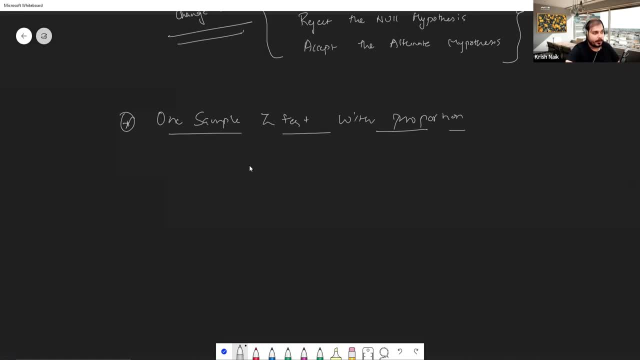 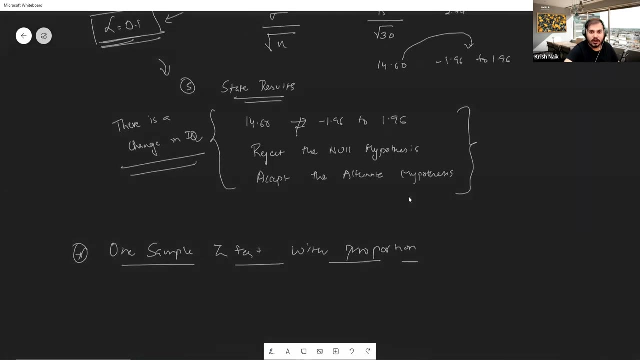 So for that you have to go with one tail or two, One tail test, okay, I'm sure. Okay, guys. So let's go with the next test, which is called as one sample Z test with proportion, Amar In this particular case, C in this particular case. here you will obviously be able to understand right. 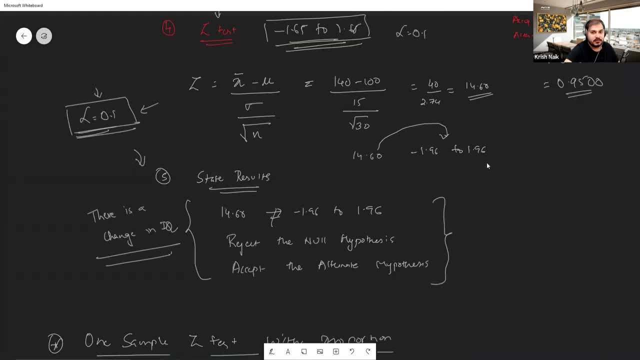 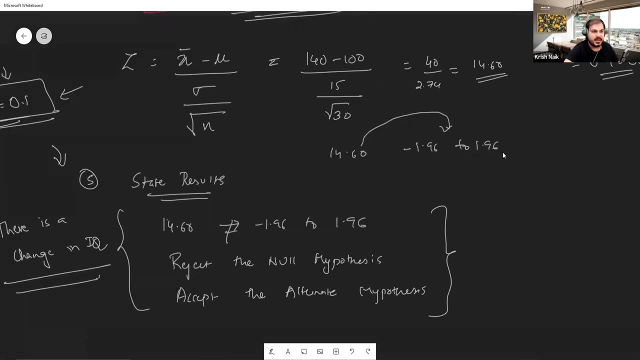 14.6 is greater than 1.96, right, Then can't you say that, okay, it will be a positive one? Very simple, no, 14.6 is greater than 1.96, right, It is not 2.. 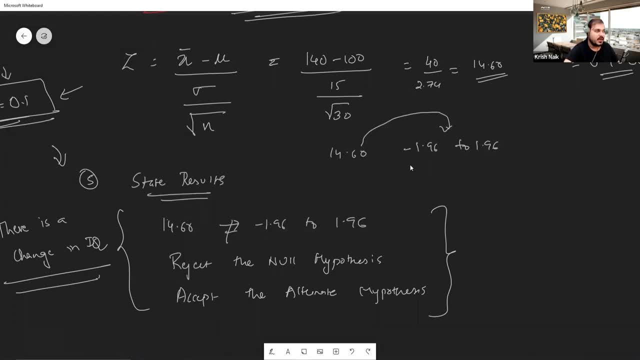 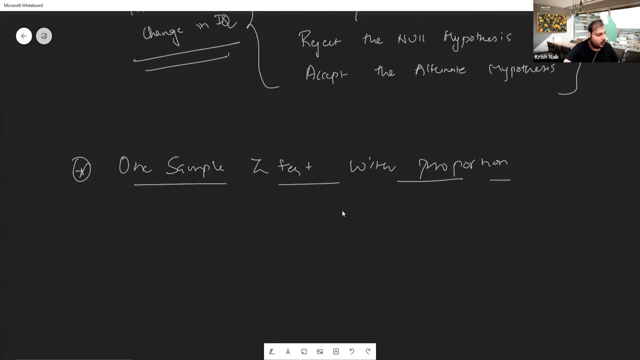 Towards minus values. If it is coming towards minus value, then you say there is a negative change. Very simple, just from seeing the data you will be able to understand. Okay, guys, Write down the problem statement. So the problem is that a survey claims that 9.9.. 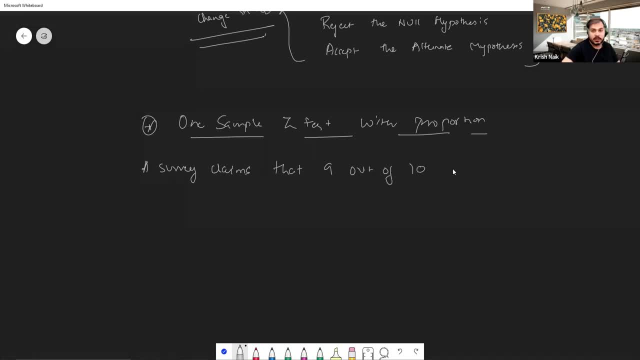 10 doctors recommend recommend aspirin: aspirin for their patients- patient with headache with headache. to test this claim, a random sample of hundred doctors is taken. out of this hundred doctors, 82 indicate that they recommend aspirin. out of this hundred doctors, 82 indicate that they recommend aspirin. 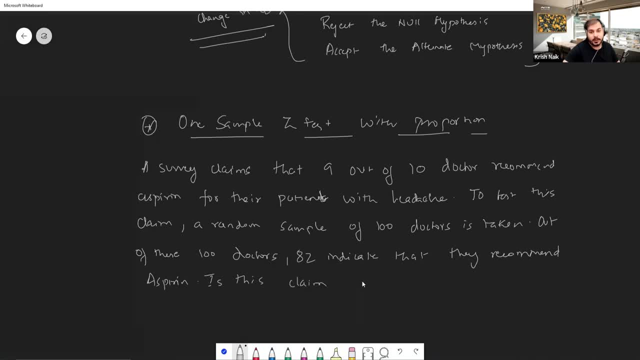 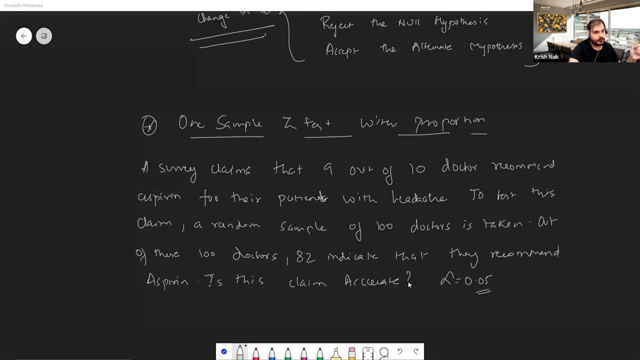 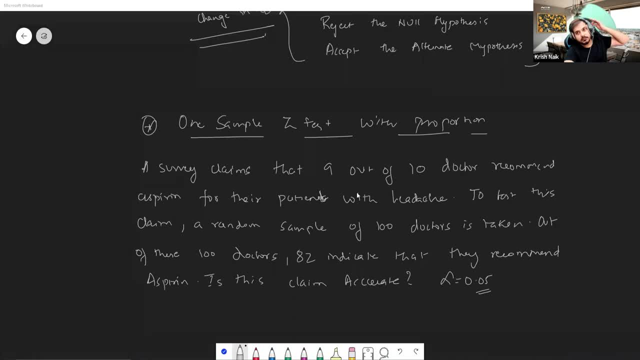 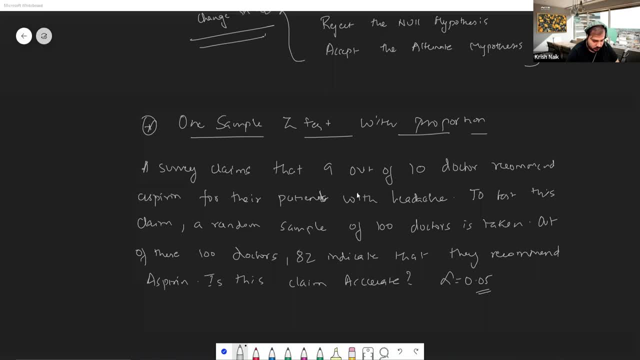 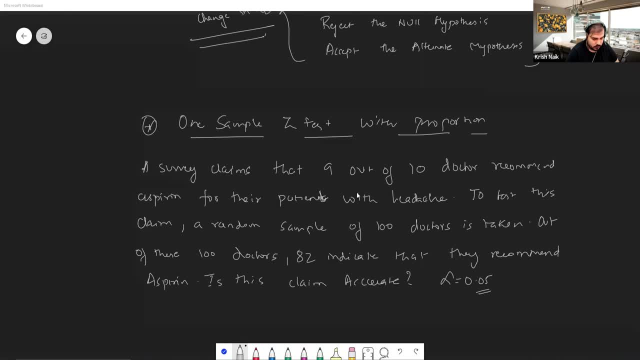 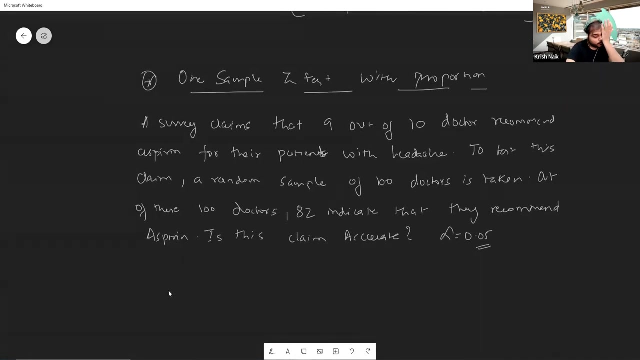 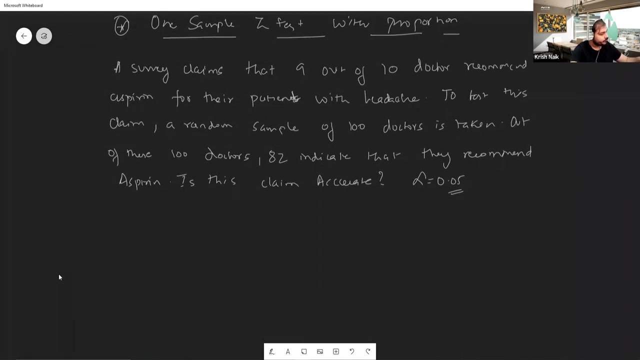 Thank you. Thank you. I'll talk about the formula. Don't worry, Everybody have written this particular thing. guys, Yes Shall I start. Okay, Now tell me what will be your null hypothesis. What will be your null hypothesis? 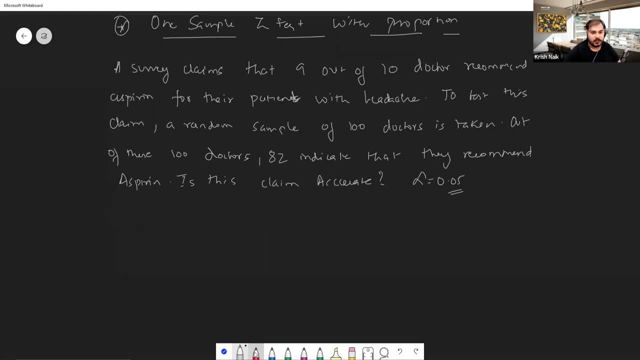 Think over it, guys, Come on. So let's start. First of all, let's define our null hypothesis. Our null hypothesis basically says that what we are testing- see a survey claims- 9 out of 10 doctors recommend aspirin for their patient. 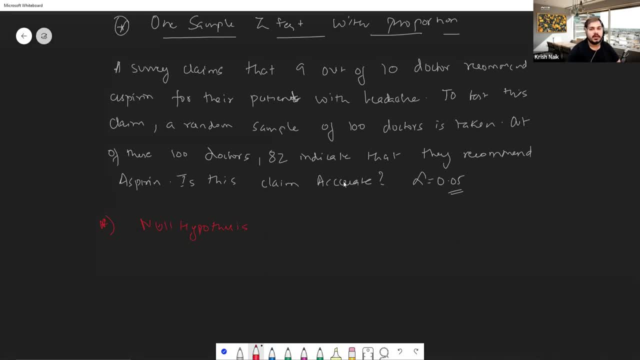 And at the end we are saying that is this claim accurate or not? right through some values, So obviously my null hypothesis will be F0. Which is nothing but P. I'll say this has P, which is my probability, which is nothing. 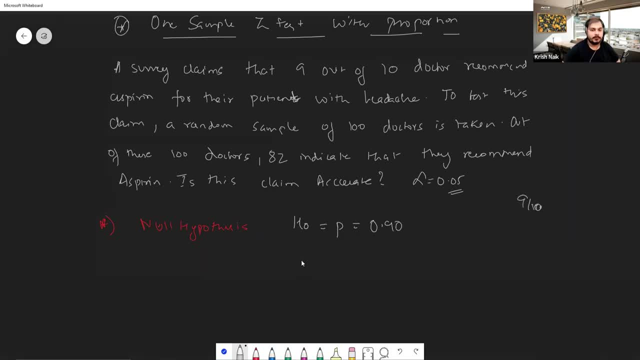 but 0.90.. Why 9? 0? 9 divided by 10.. Okay, And my alternate hypothesis will be not equal to 0.90.. Okay, Clear Anybody. This is my null and this is my alternate. 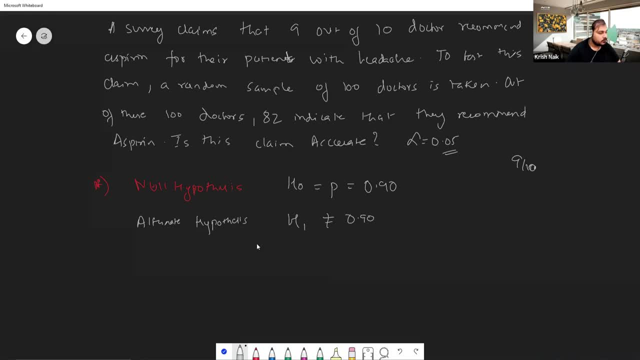 Okay. So I'm going to say, I'm going to tell you guys what I am working on. What is the difference between what I am working on and what I am not working on? So I have my null hypothesis and my beneficiary. So I have a null hypothesis. 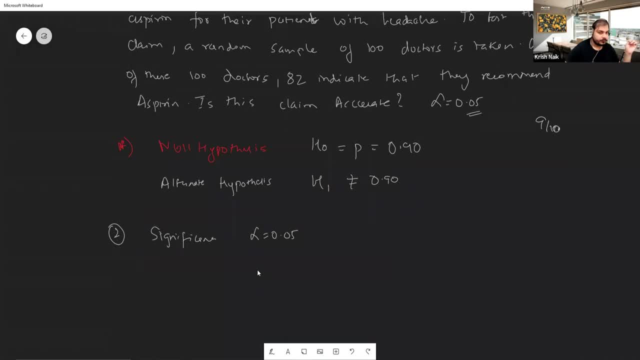 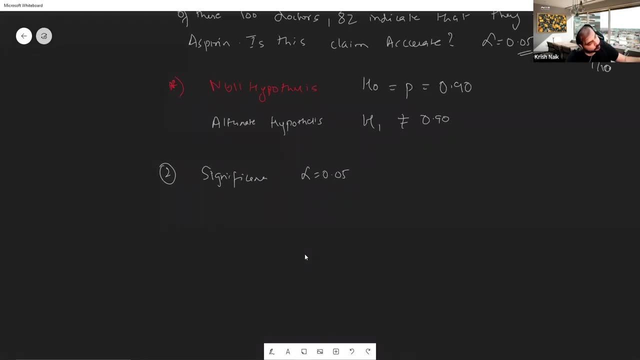 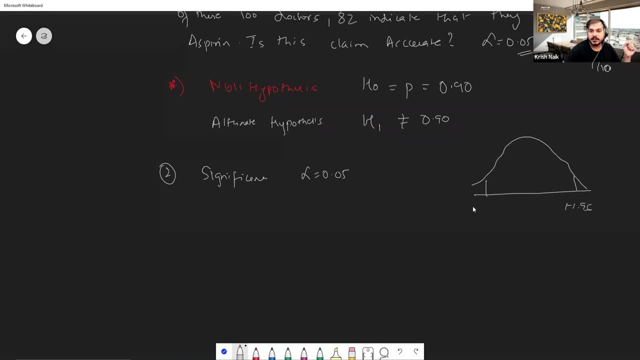 plus 1.96 minus 1.96. okay, so this will obviously be my range. because my alpha value is 0.025, i'll subtract 1 minus 0.025, it will be nothing but 0.9750. i'll go and see in my z table, okay. 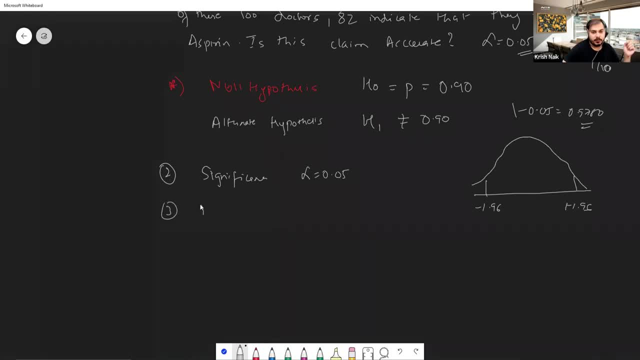 so i have got the range. so in the third step my decision rule is also done. first step: i will try to apply this particular z statistics now. here your formula will change, guys. whenever a proportion is given, you have a different formula to do the z statistics. so here i'm just going to write z 0. just see the formula: p bar minus p 0 divided by: 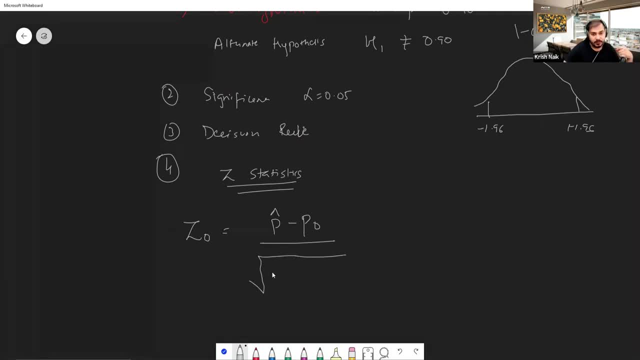 again, guys, i'm not going to derive this because this has already been proved: p 0, 1 minus p 0 divided by n. okay, now let's understand what is this p bar? p bar is nothing, but it is the probability with respect to the sample. 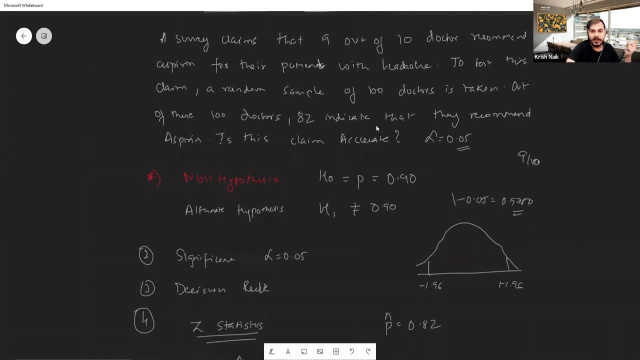 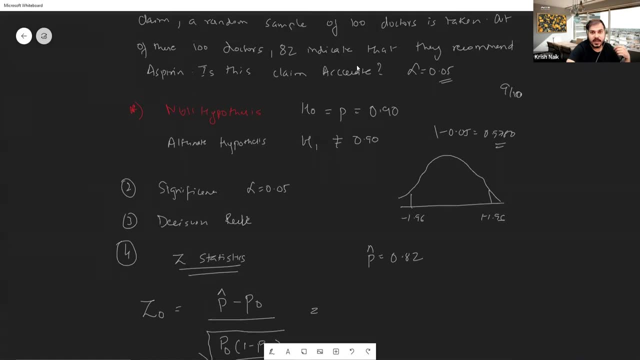 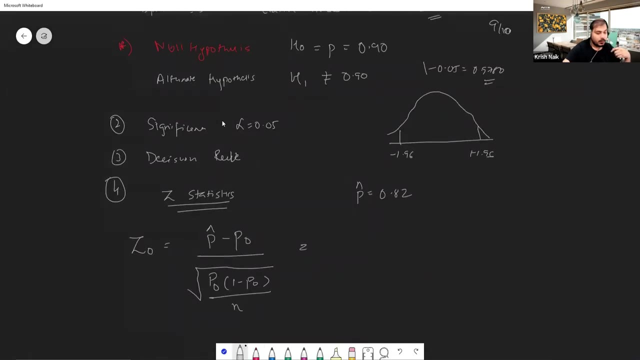 that is given. so it is 0.82. see over here it says 82 indicate that ray recommends aspirin out of 100. so this will be my p bar. p 0 is basically my this sample that is given with respect to the population: 9 out of 10. right, so my p 0 is nothing but 0.90. and then x is: 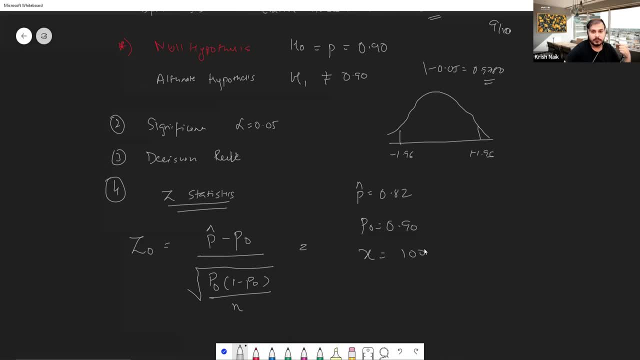 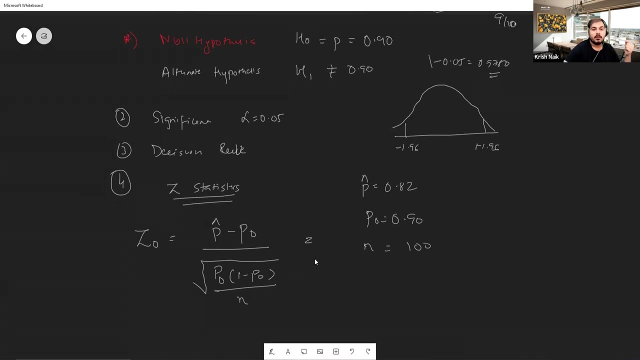 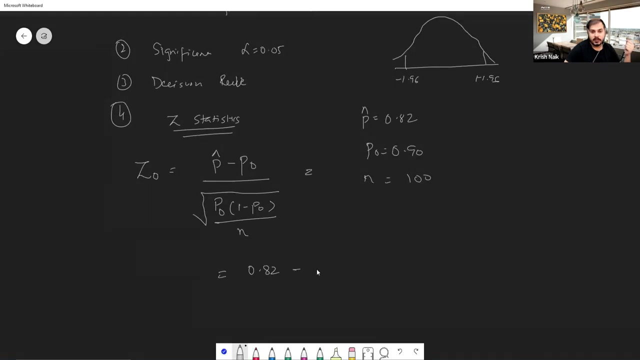 nothing but 100. this is basically my sample. okay, x is nothing but my sample. or i can also say this as small n, small n. okay, now let's go and compute this formula. now computing: i'll get 0.82 minus 0.90 root of. 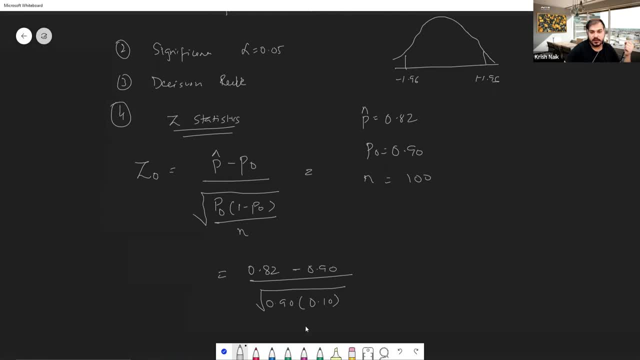 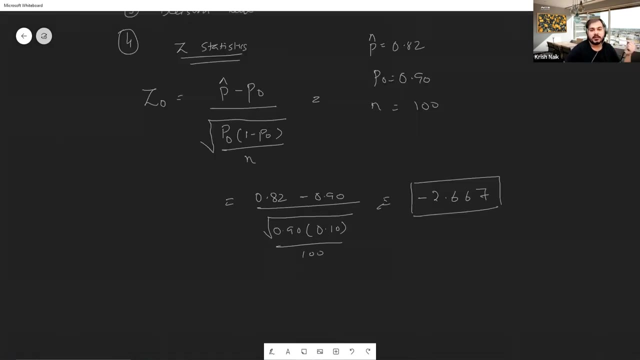 0.90 multiplied by 0.10, divided by 100, if i do this computation, my computation will be 0.90, will be somewhere around minus 2.667. now tell me, from this particular value should we reject or accept the null hypothesis? 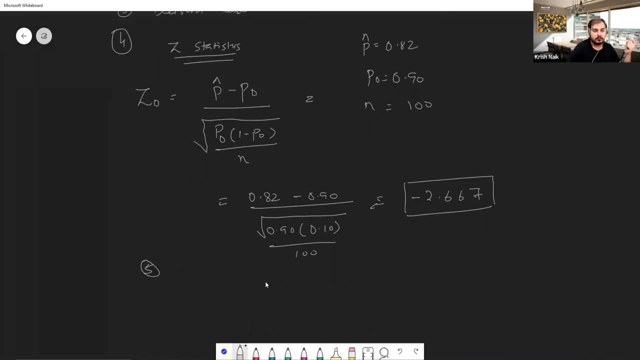 should we reject or not accept the null hypothesis? you should reject the null hypothesis because, see, it is less than it is. it is less than 1.96, right, minus 1.96. okay now just imagine, guys, if my output was coming like this, then what we have to do. suppose if my output was like this: 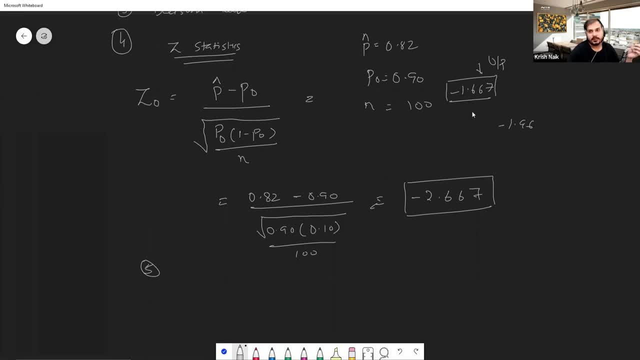 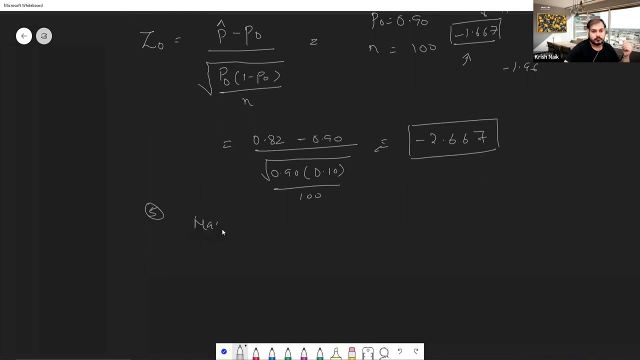 then we should we reject or accept, accept the null hypothesis, right, perfect. so here, finally, we make some conclusion, make some conclusion here saying that minus 2.667 does not fall in the range between minus 1.96 to 1.96. so we reject the null hypothesis. 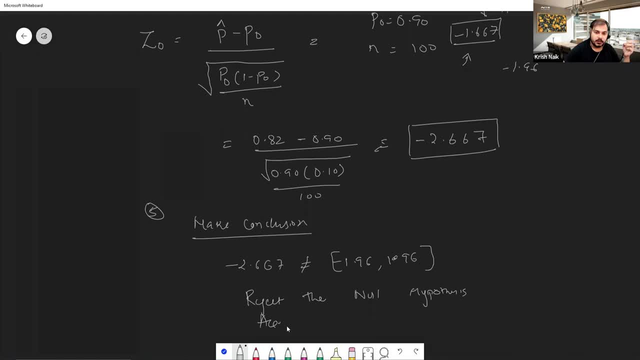 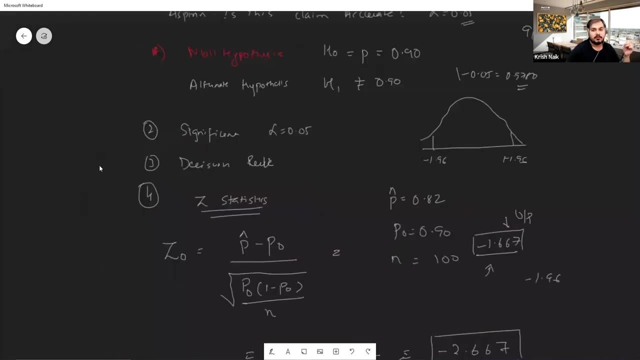 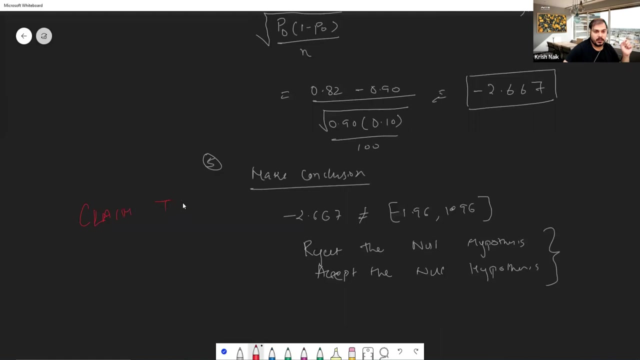 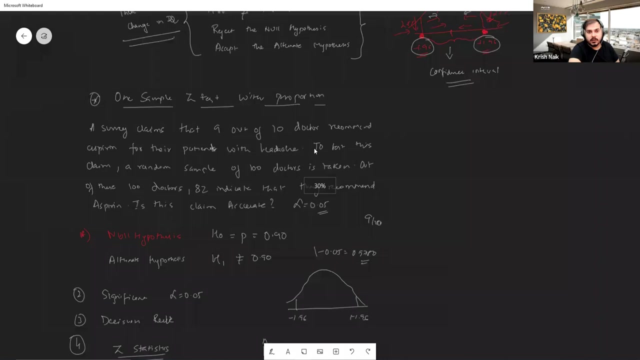 and we accept the null hypothesis. that basically means what that basically means. what that basically means: this claim is inaccurate, and here you have the proof why it is inaccurate. okay, guys, so i hope you like this session and, yes, we will continue the things in the next session itself. 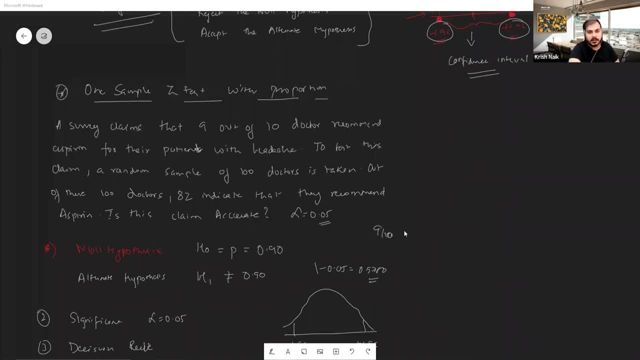 in the next session we'll try to see some practical part and probably i hope you liked it. if you liked it, don't forget to, you know, go and put some amazing reviews on inuron in the google review itself, right? so thank you one at all. i'll see you all in the 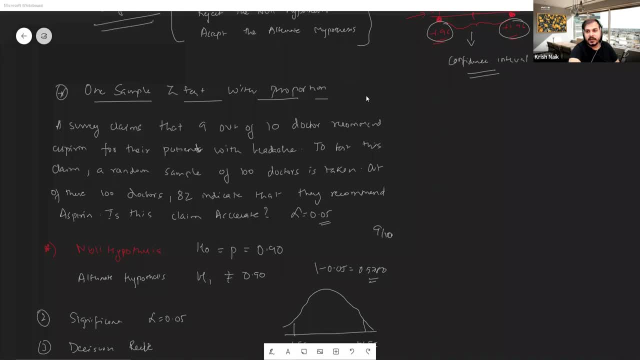 next session. have a great day ahead and keep on rocking, keep on learning and in the next session we'll be having practical implementation. thank you guys. bye.